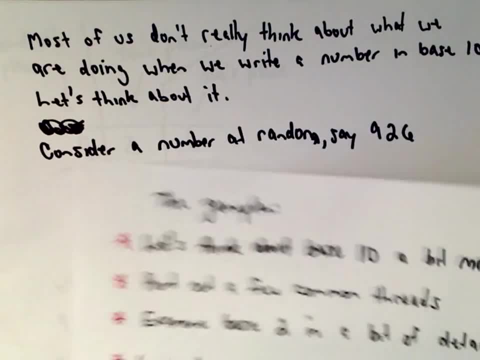 So we'll just do some basic examples. Okay so, Okay. so here we go. Okay, so you know again. I don't really think most of us really think about what we're doing when we write a number in base 10.. 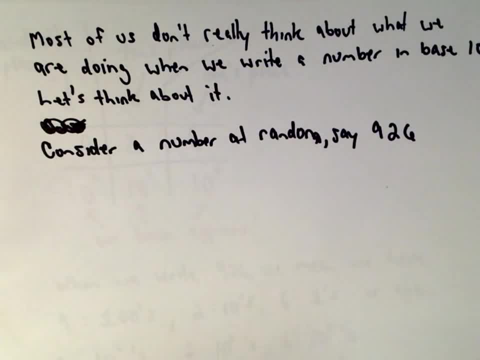 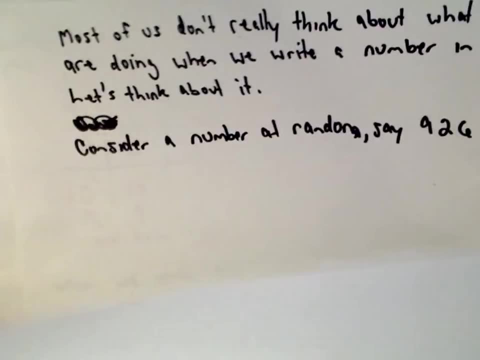 You know, if we write the number 926, what does that mean? Well, it means, right, you have 926 things. So, okay, that's a little redundant, right? But let's really look at what we're doing. 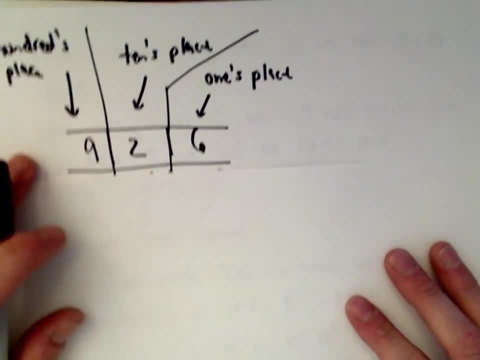 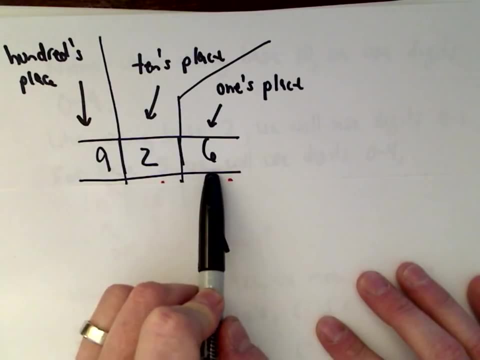 So let's look at that number: 926.. So of course you know this is stuff you see in elementary school. The 6 is what we say. That's in the ones place. The 2 is in the tens place. 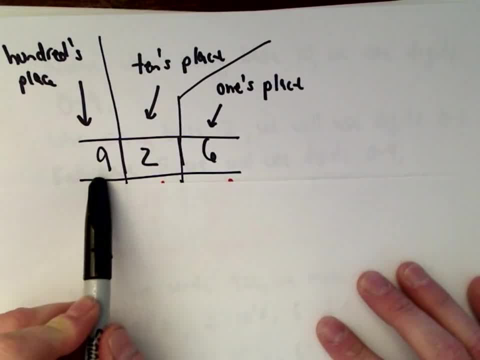 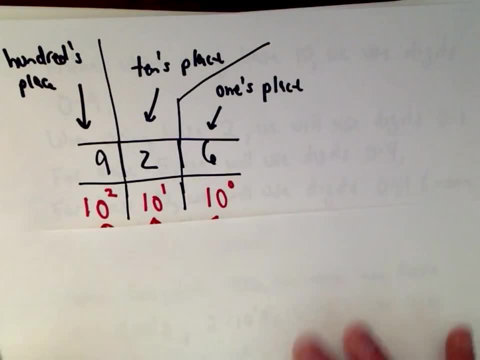 And the 9 is in the hundreds place. right, We have 9 one-hundreds, 2 tens and 6 ones, And if you think about it, we can write, you know, the hundreds as nines, The hundreds as our base, which is 10.. 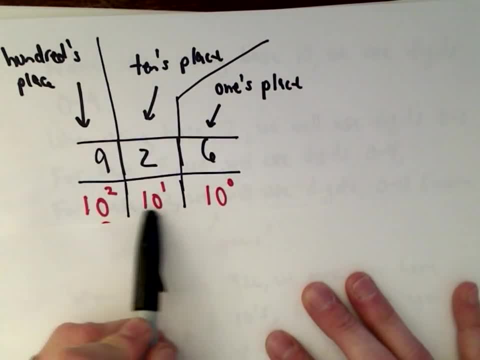 10 to the power of 2.. We can write the tens place Well, that's our base, which is 10 to the power of 1., And the ones place well, 1, that's just 10 to the power of 0.. 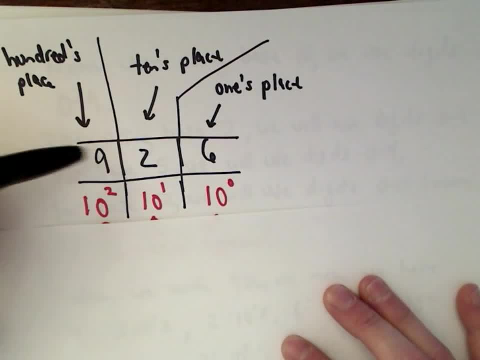 And we're going to see this theme crop up over and over again, And that's why I'm kind of pointing it out. The columns are going to represent the base raised to the exponent of 0.. The base, excuse me, yes, the base raised to the exponent of 1.. 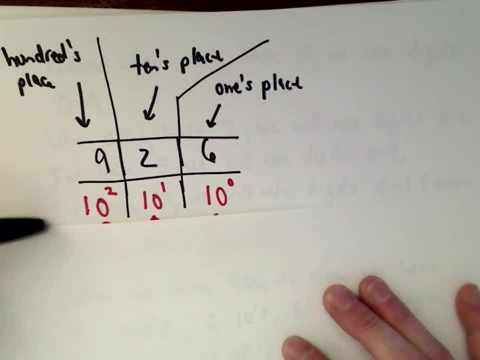 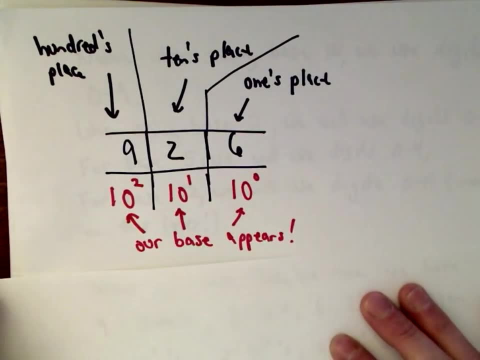 The base raised to the exponent of 2,, etc. The base raised to the exponent of 3,, if you have a larger number, And so, again, our base is appearing here. That's what I'm trying to point out And what I said just a second ago. I want to say that again. 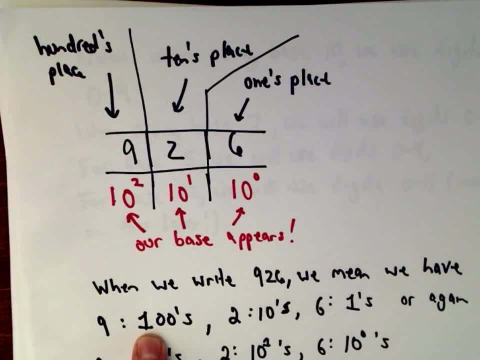 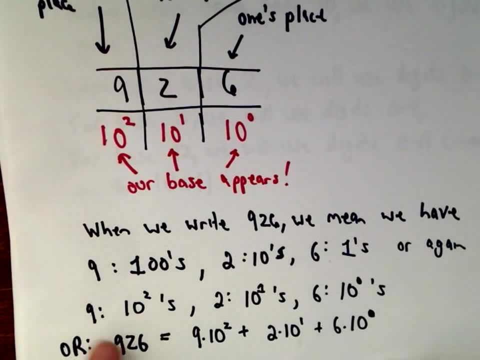 The number 926,. what does that mean? Well, it means we have 9 one-hundreds, We have 2 tens, We have 6 ones, Or again, writing this, using our base, we have 9. of our base, 10 to the power of 2.. 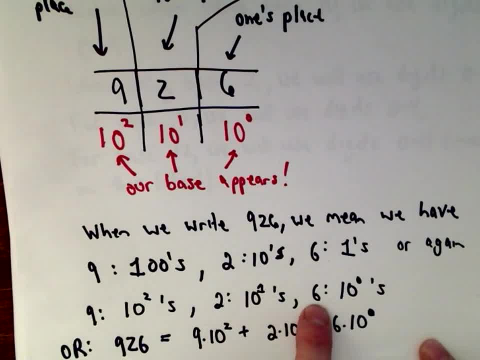 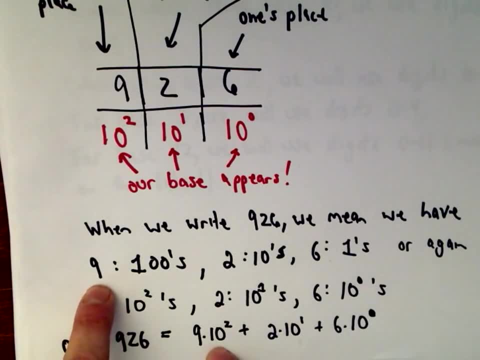 We have 2 of our base 10 to the power of 1.. And we have 6 of our base 10 to the power of 0. And when we mean 926, what it means is we take: well, we have 9 one-hundreds, which is 9 times 10 squared. 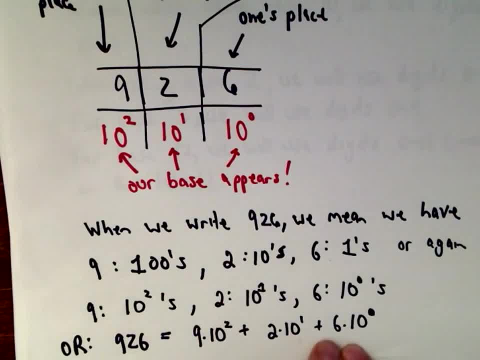 We have 2 tens, which is 2 times 10.. And we have 6 ones, which is 6 times 10 to the 0 power, And if we add those together we get 926.. That's what we mean when we write the number 926. 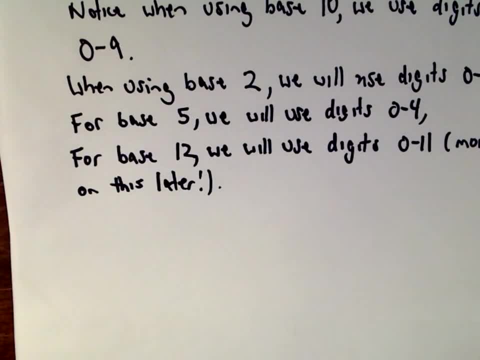 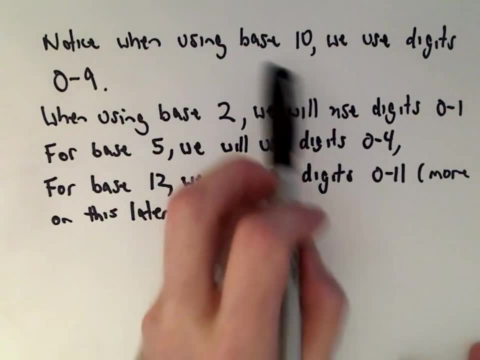 Okay, you're like: alright, Patrick, I know this, So let's look at this. We'll start looking at base 2 here in just a second, But I want to point out something real quick. So when we use base 10, we're only using the digits 0 through 9, right? 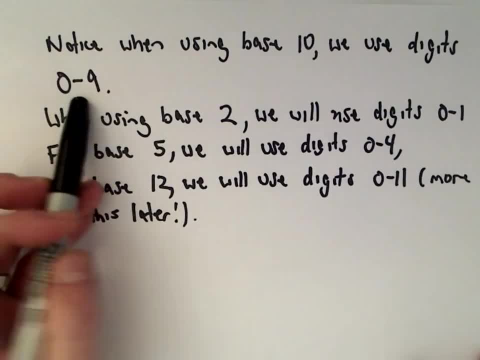 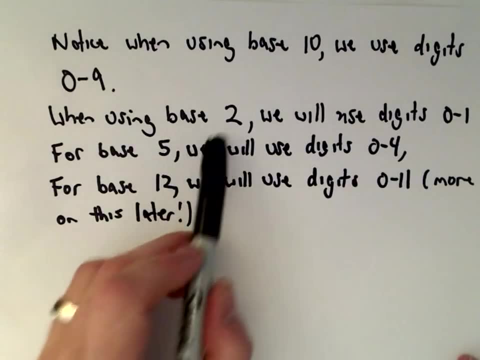 Those are our symbols that we use: 0 through 9.. When we write a number like 10, well, we're really just using the digits 1 and 0. When we use base 2, we're only going to use the digits 0 to 1.. 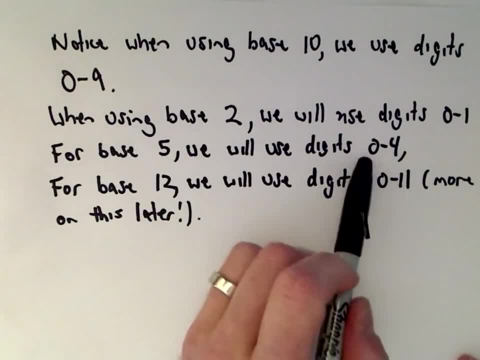 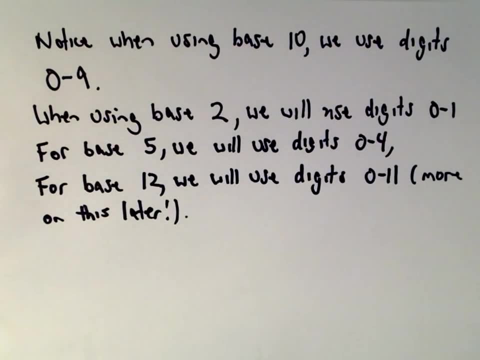 And for example, for base 5, well, we're only going to use the digits 0 through 4.. Now, my last one's really not quite true, but hopefully you'll get the gist of what I'm saying here. 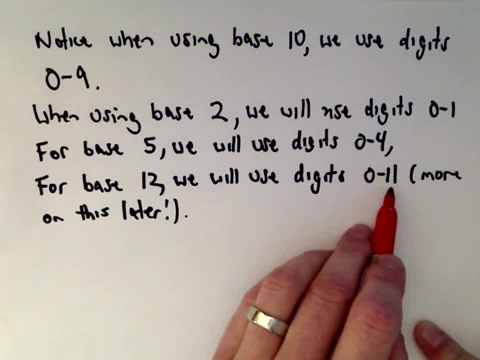 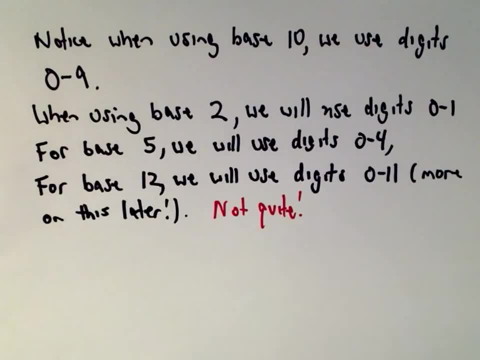 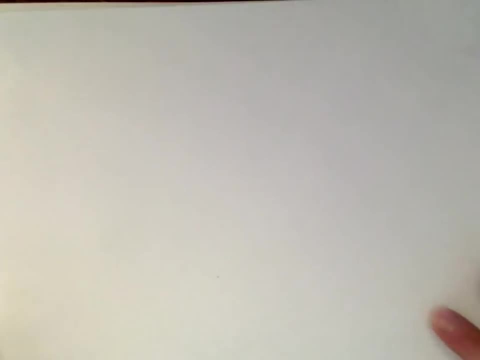 For base 12, we'll use the digits 0 through 11.. Well, not quite. We're going to have to introduce some new symbols for that. We'll see here in a moment. But let's just make up some random examples here of numbers in different bases. 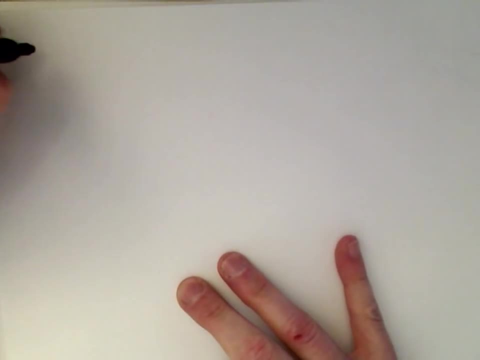 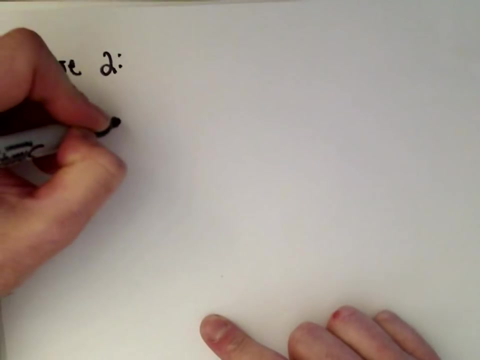 And then we'll just convert back and forth. Let's look at something using base 2.. So let's look at the number. Let's just say I'm going to make a number at random, So let's do 1011.. 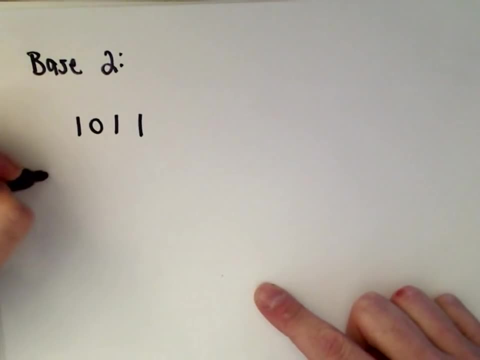 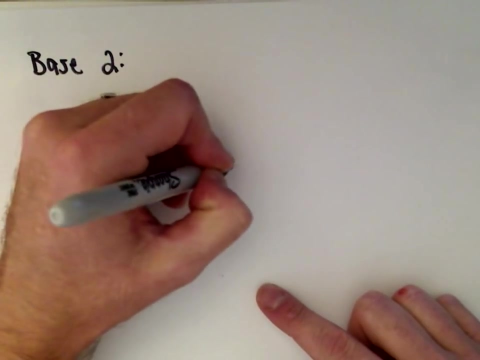 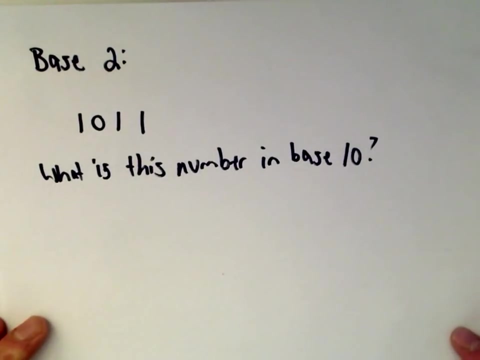 So if this is in base 2, what number? So I want to know what is this number in base 10.. And base 10 is also called decimal. So we could say: what is You know? if this number 1011 is in base 2, what is this number in base 10?? 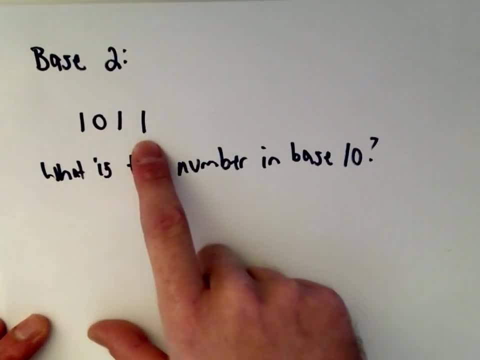 So suppose a computer right, Computers just use 1s and 0s. If a computer ran across this and would want to interpret it, If we wanted to interpret it as a number in base 10, what number is that? 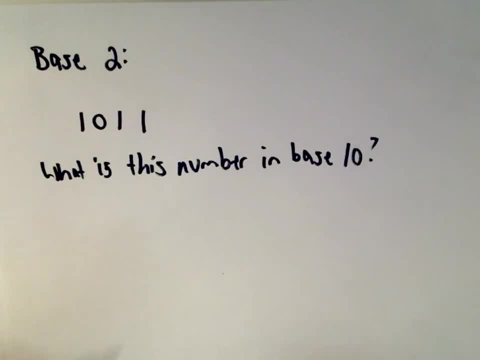 Well, again, what you can think is Okay. so here's our number 1.. I'm going to just make a little column, like a second ago: 0,, 1, and 1.. Well, let's think about our base. 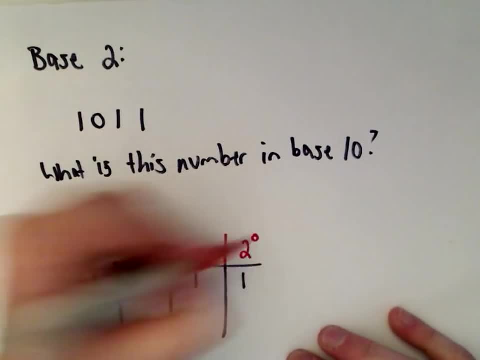 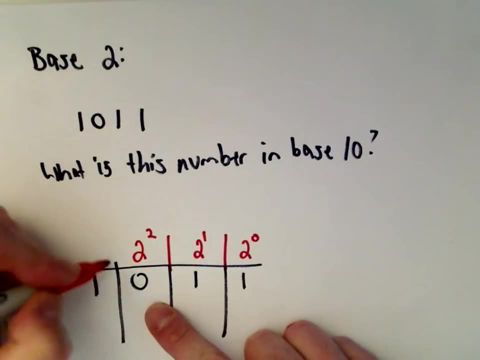 Okay, again, we're using base 2.. So this is going to be 2 to the 0.. This is going to represent 2 to the 1st power. This is going to represent 2 to the 2nd power. 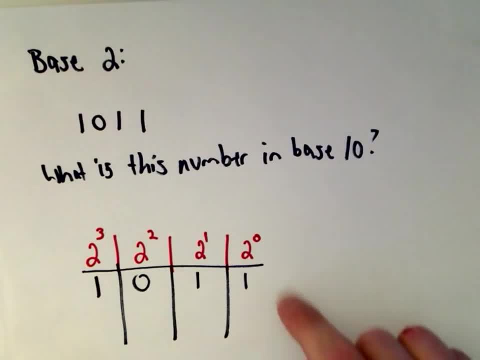 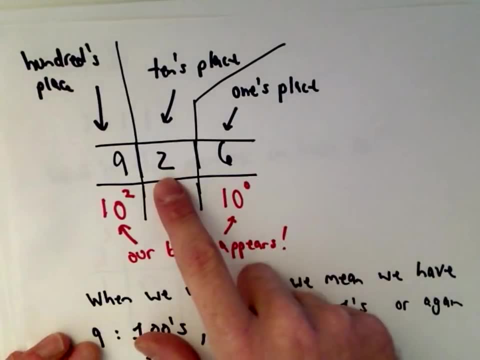 And this is going to represent 2 to the 3rd power. So we don't have just like a second ago- right A second ago- we had the 1s place and the 10s place and the 100s place. 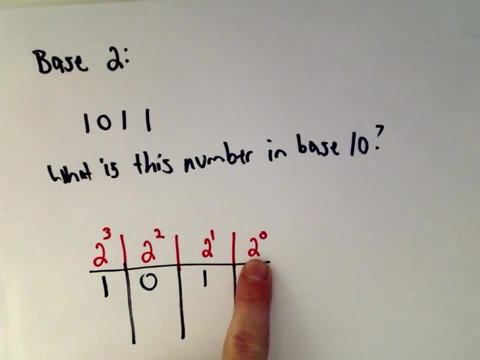 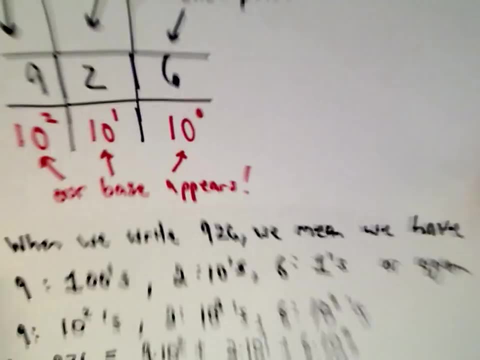 We don't have that anymore. Now we have the 1s place and the 2s place and the 2 squareds place and the 2 to the 3rd powers place, And what we'll do is we just do the same thing. 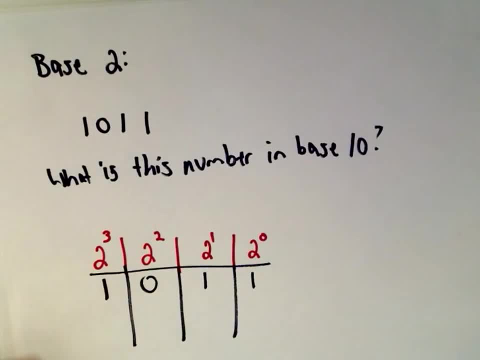 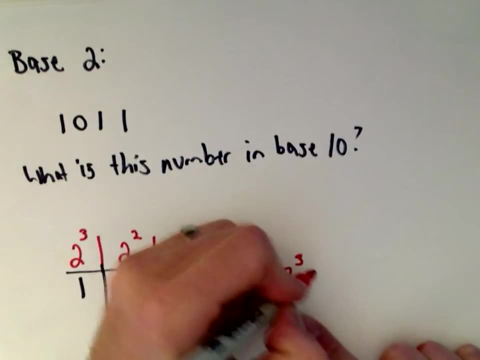 We basically just add those numbers together. So this number 1011, it says really we have 1 times 2 to the 3rd. So we have 1, 2 to the 3rd, Plus we have, well, 0 of the 2 squareds. 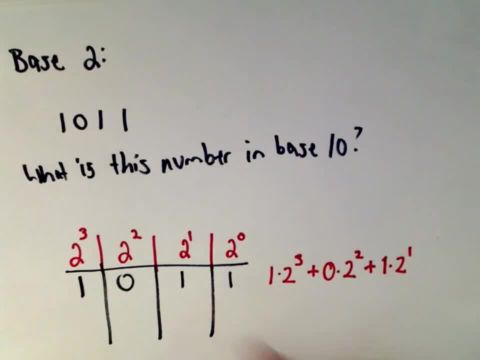 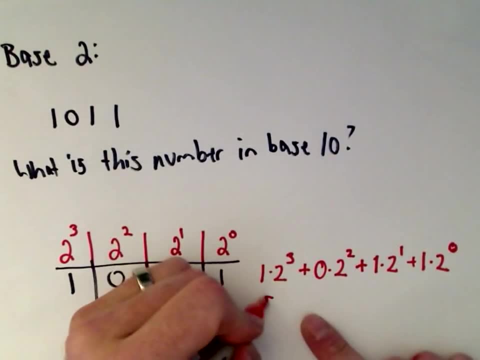 We have 1 of the 2 to the 1sts, And then we have another 1 of the 2 to the 0s. Well, if we convert that, well, 2 to the 3rd, that's 8.. 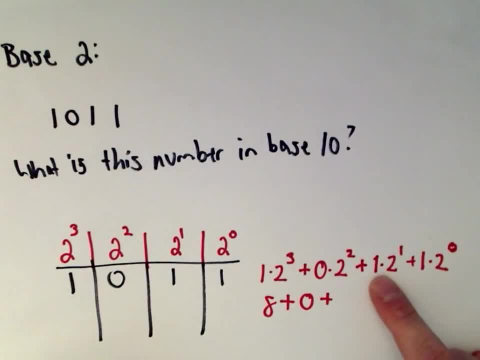 Well, 0 times anything is 0. We'll have 1 times 2, which will be 2.. We've got 1 times 2 to the 0. That'll be 1 times 1 or 1.. So 8 plus 0 plus 2 plus 1.. 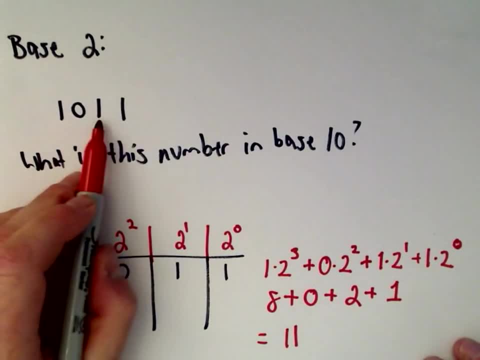 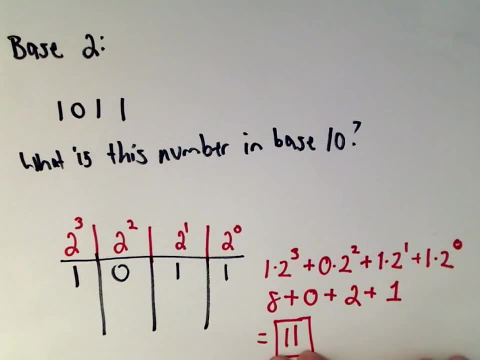 That's going to be the number 11.. So the number 1011, that's going to equal the number 11 in base 10.. Likewise we could write the number 11.. If somebody said: you know how do you write the number 11 in base 2?? 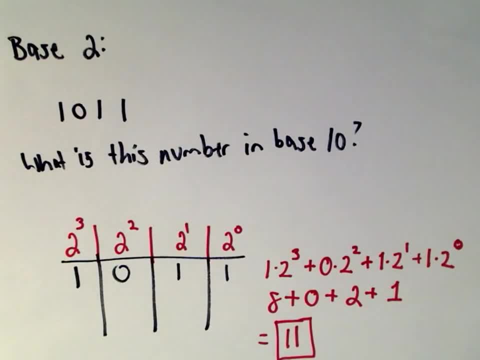 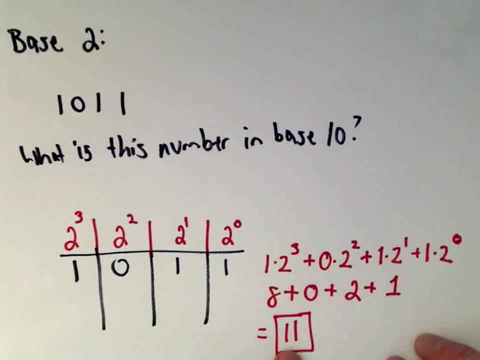 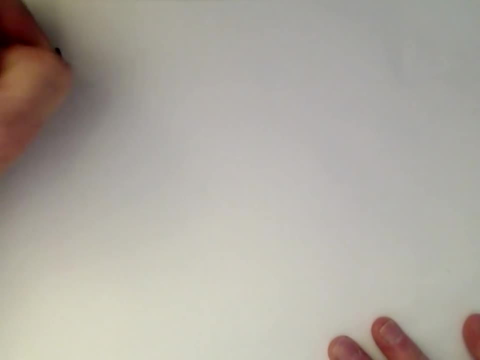 Well, it would be 1011.. So let's show how to convert, you know. Let's look at an example of taking a number in base 10 and rewriting it in base 2.. So let's write the number 11.. 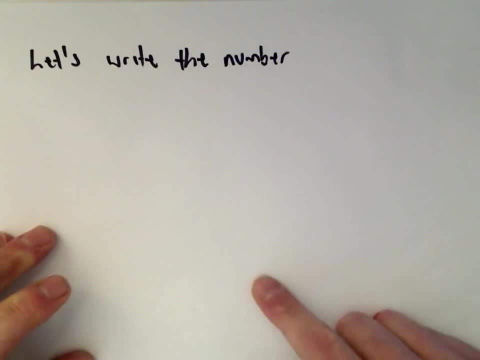 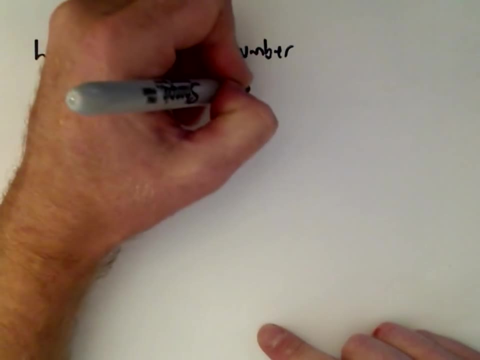 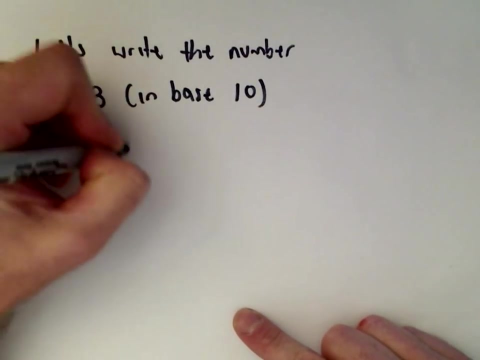 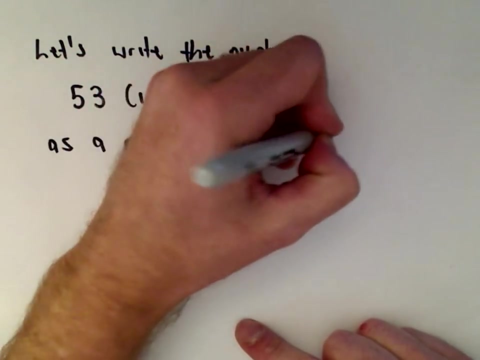 And again I'm just making up a number at random here. Let's look at the number I don't know, 53. And we're going to assume this is in base 10.. So let's write the number 53,, which is in base 10, as a number in base 2.. 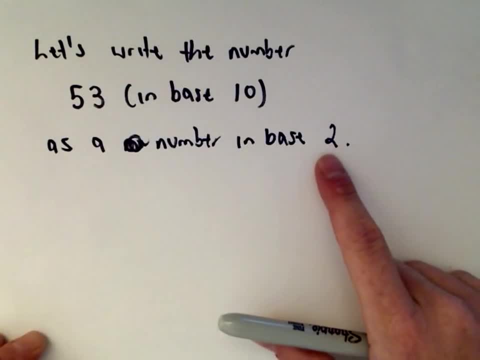 Okay, so what you want to do is you want to find the largest power of 2 that would go into 53 without going over. So that's going to be the first sort of game plan here. So let's write down some powers of 2.. 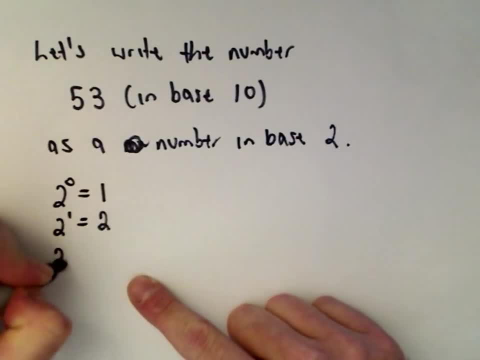 Well, 2 to the 0, we said that's 1.. 2 to the 1st, that's 2.. 2 squared that's 4. 2 to the 3rd power, that's 8.. 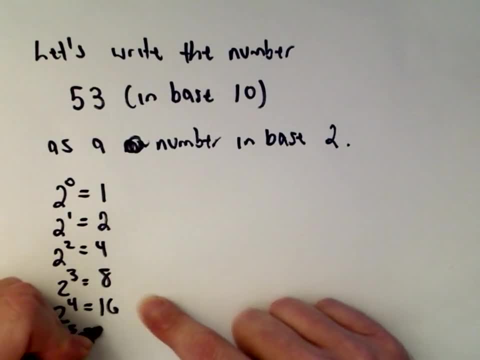 2 to the 4th power, that's 16.. 2 to the 5th power, that's going to be 32.. And 2 to the 6th power, that's going to be the number 64.. 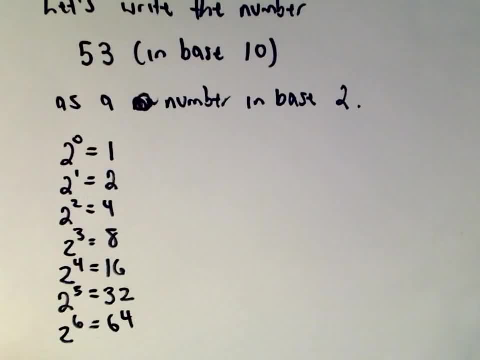 So let me give myself a little more room here. Okay so the largest number that would go into 53, the largest power of 2 would be 2 to the 5th power. Okay so, let's see, So we've got 53.. 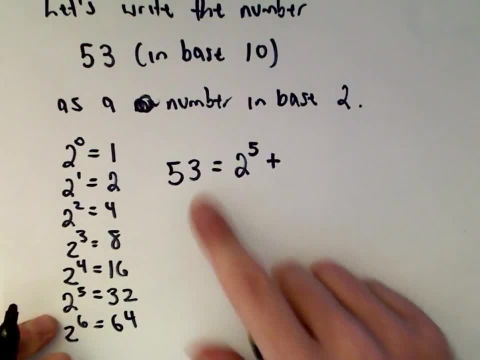 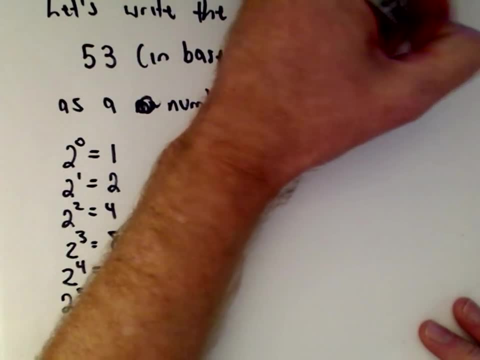 We can write that as 2 to the 5th power. Okay, well, 2 to the 5th power. we said that's 32.. So let's see 53 minus 32.. That's going to leave us with 21.. 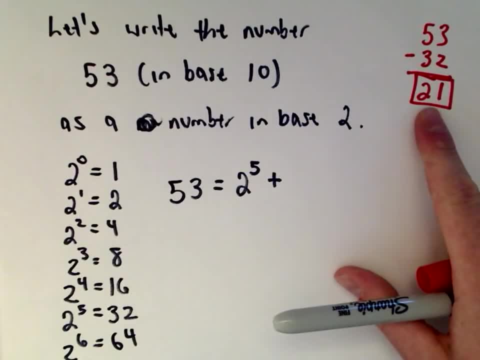 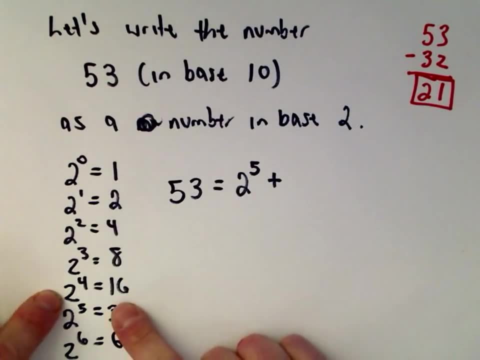 And now we do the same thing with this remainder. We think what's the biggest power of 2 that will go into 21 without going over? Well, it looks like okay. 2 to the 4th, that's 16.. 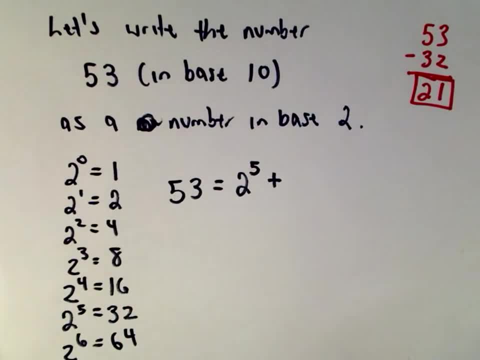 Again, 2 to the 5th is too big. So if we use 2 to the 4th, okay. so now I've got the number So far, I've got 32 plus 16.. Well, again okay if I take 21 and I subtract away 16,. 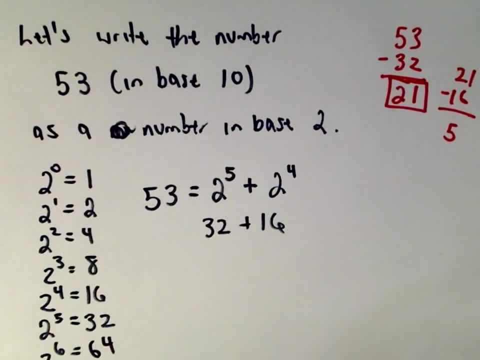 that's going to leave us with 5 remaining. So I'm going to do the same thing. I'm going to think what's the biggest power of 2 that will go into 5 without going over? Well, 2 squared. 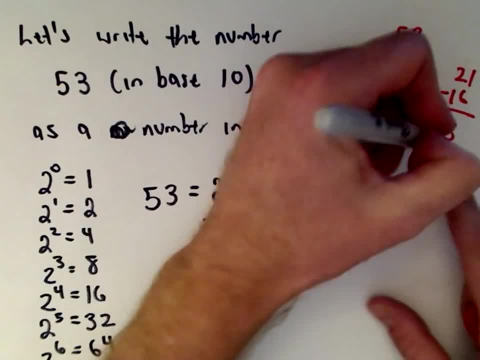 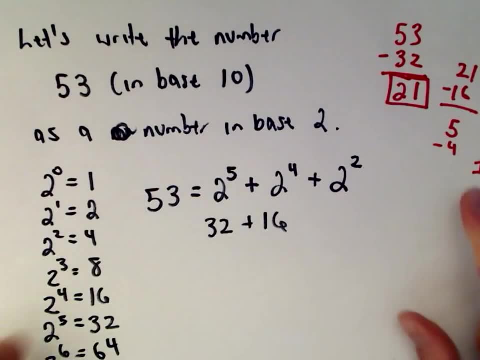 2 squared is going to give us 4.. So again, we can subtract away 4.. So now we've just got 1 left over. Well, the largest power of 2 that would go into the number 1 without going over would be 2 to the 0.. 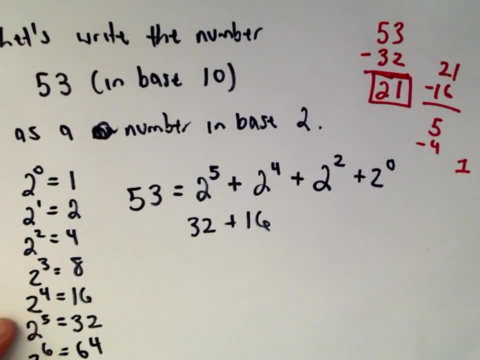 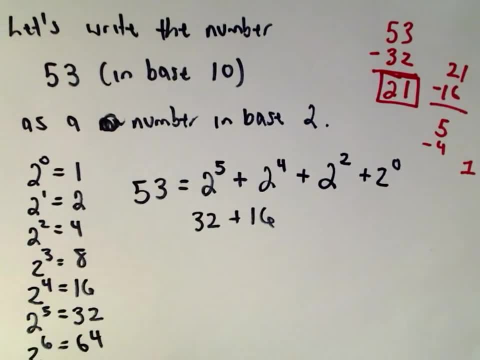 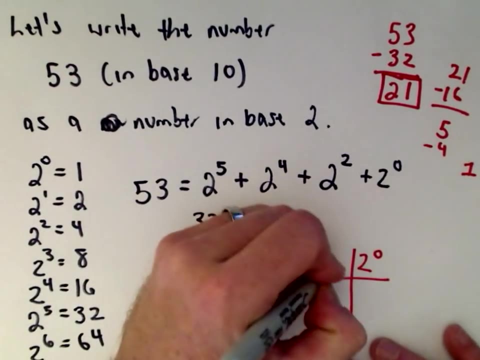 2 to the 0.. 2 to the 0 power. So just like a second ago, if you think about, you know making this little column, So I'm going to make one of these here. So we've got 2 to the 0. 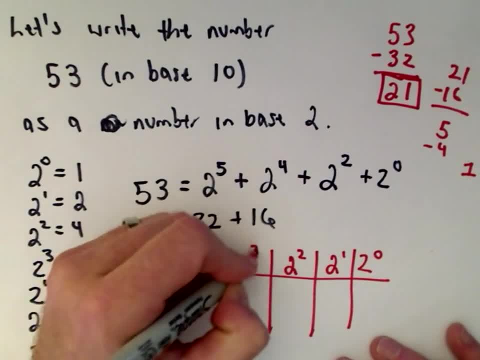 We've got 2 to the 1st, We've got 2 squared, We've got 2 to the 3rd, We've got 2 to the 4th And we've got 2 to the 5th. 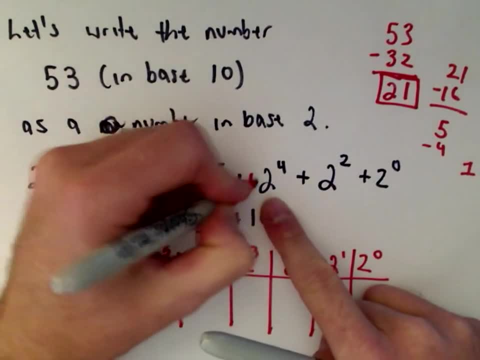 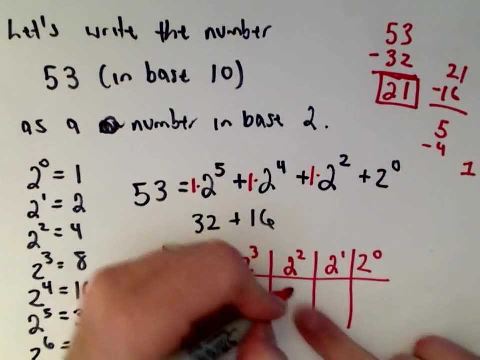 Well, let's see, We've got 1, 2 to the 5th, We've got 1, 2 to the 4th. We have 0, 2 to the 3rd powers. We have 1 of the 2 squares or 2 to the 2nd power. 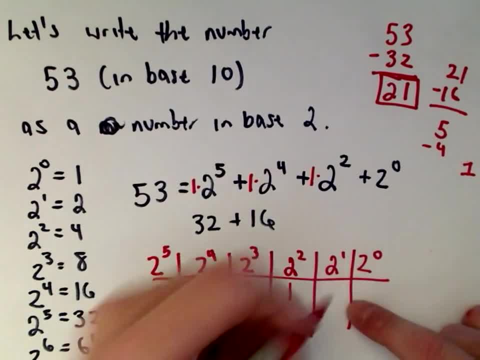 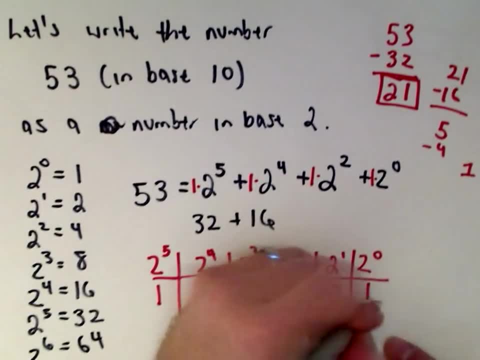 There's no term involving 2 to the 1st power, So we've got 0 of those And, last but not least, we have 1 of our base 2 to the 0. That's going to be the number 53 now in base 2.. 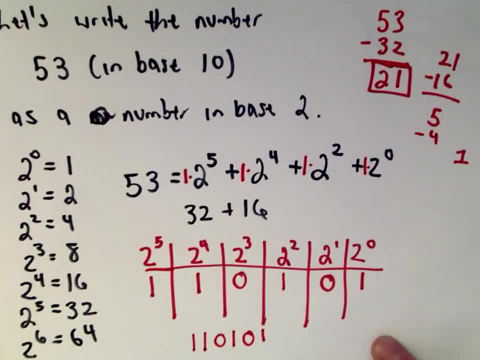 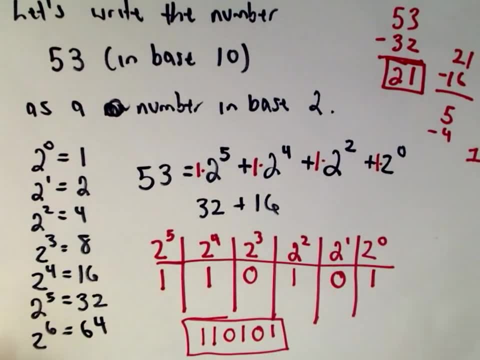 It's going to be the number 110101.. That would be The base 2 representation for our familiar number 53.. Okay, So that's base 2.. That's how you go about doing base 2.. For those of you that want to see more of these: 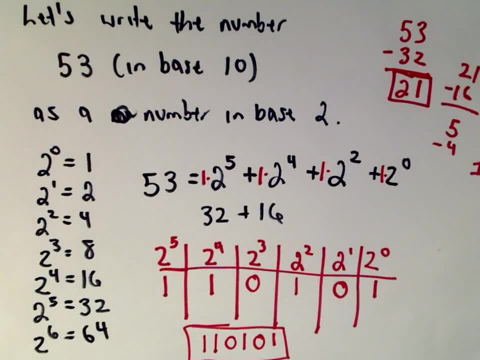 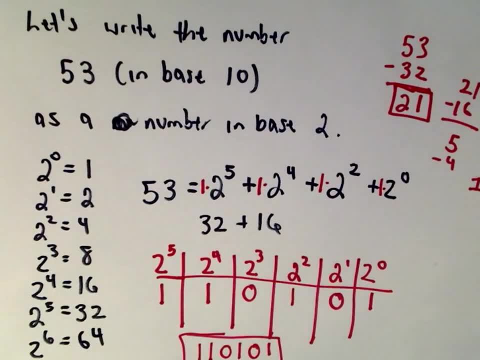 leave a comment in the video, and I'll be happy to go over some more of these, But this is the basic idea. Excuse me, So I think I said let's pick a number in base 5.. One other thing I want to point out as well. 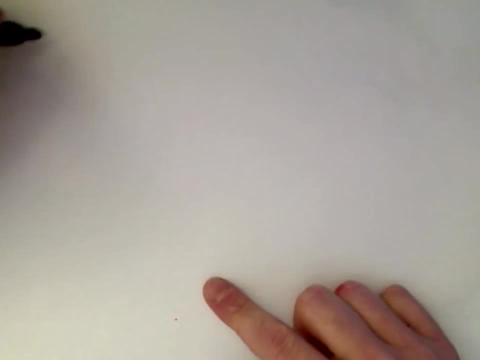 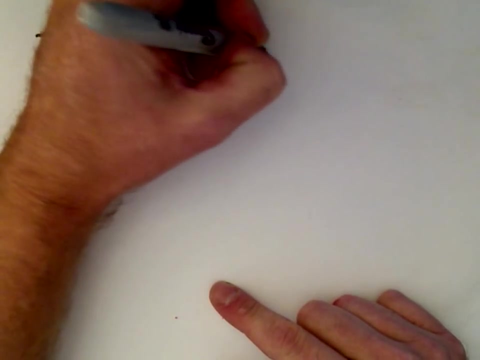 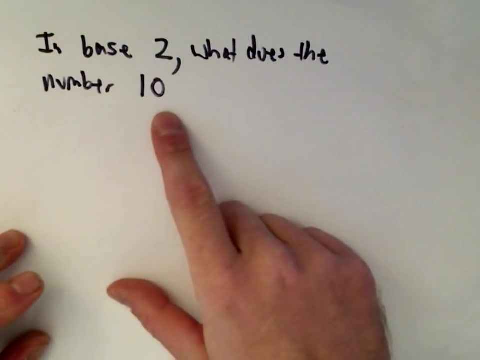 One other thing that I think is interesting: In base 2.. In base 2.. What does the number, What does the number 10 represent? Well, again, if we think about it, that means we have 0 times 2 to the 0 power. 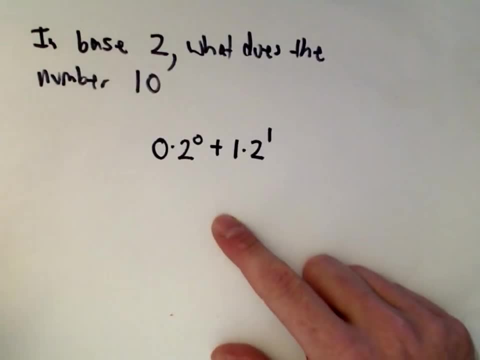 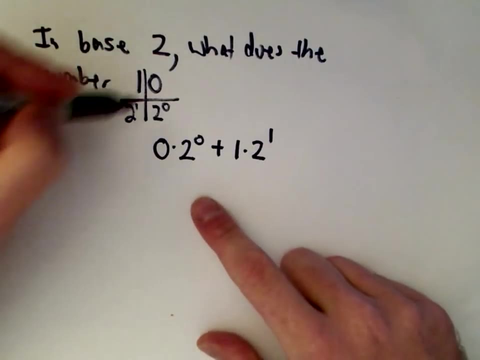 Plus we have 1 times 2 to the 1st power. So again, if you think about making our columns, this is the 2 to the 0 power, 2 to the 1st power. So it says we have 1 of the 2 to the 1st powers. 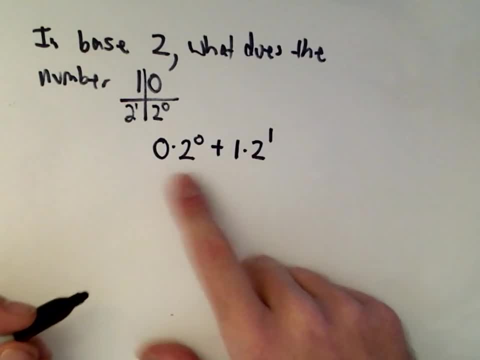 0 of the 2 to the 0 powers. Well, we get 0 plus 2.. It gives us the number 2.. No matter what base you're using, the number 10, or I shouldn't say 10,. 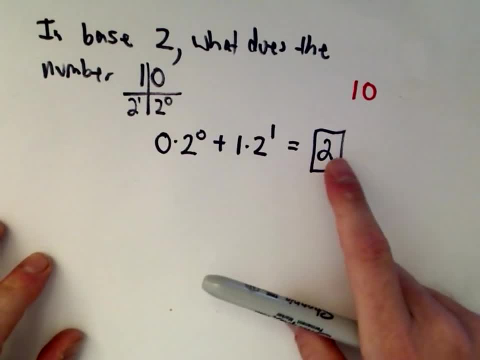 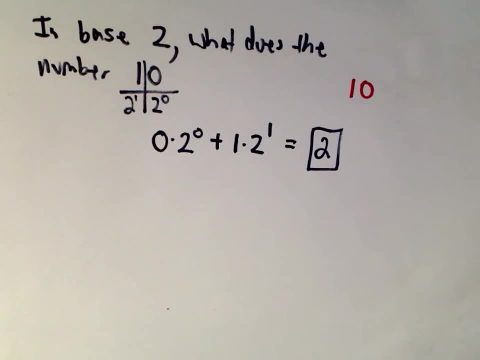 10, that's going to always represent whatever your base is. And Okay, Maybe that should be obvious if you think about it. But to me, you know, at first it just kind of That to me somehow is a very pleasing 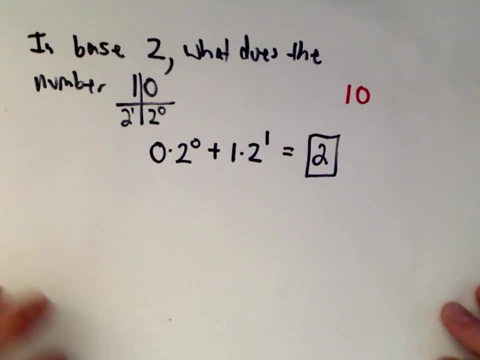 I don't know. I find it very satisfactory, Or very satisfying, I should say So. hopefully you'll find it interesting too. So I said I Let's look at a number, in base 5.. So let's do the same thing. 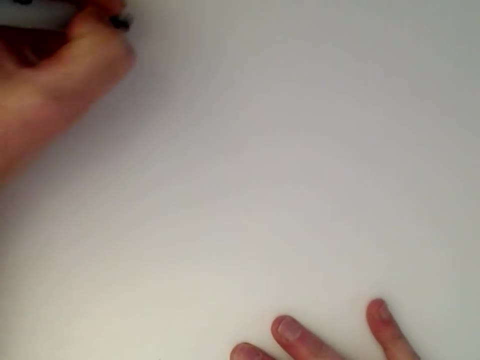 I'm just going to do one of these. Let's look at a number in. So this is a number in base 5.. So again, we can only use the digits here: 0 through 4.. So let's convert from our number that's in base 5.. 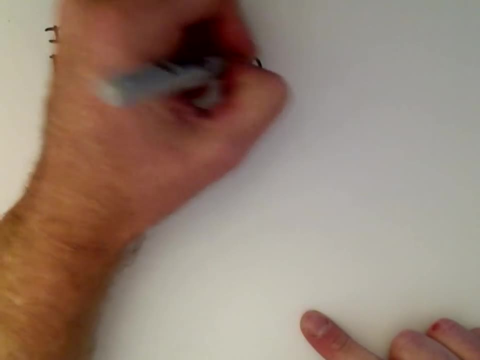 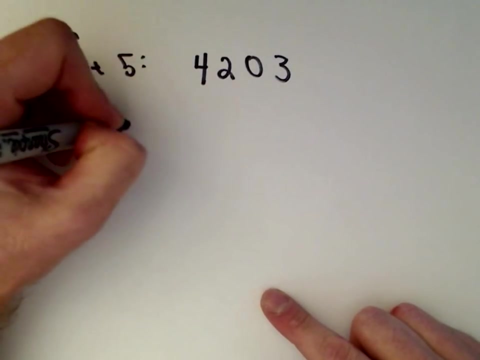 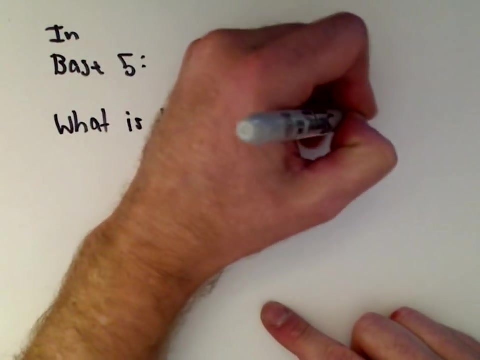 I'm going to use 4,, 2,, 0,, 3.. And I want to think: okay, so here's our number in base 5.. What is this number in base 10?? Well, again, it's just going to be the same thing. 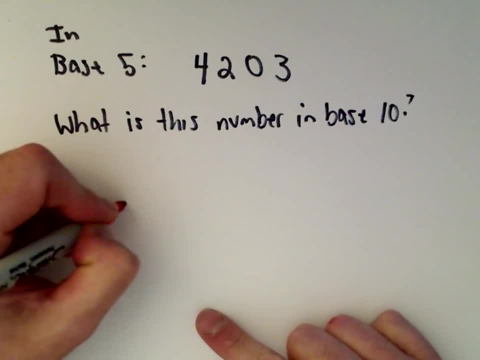 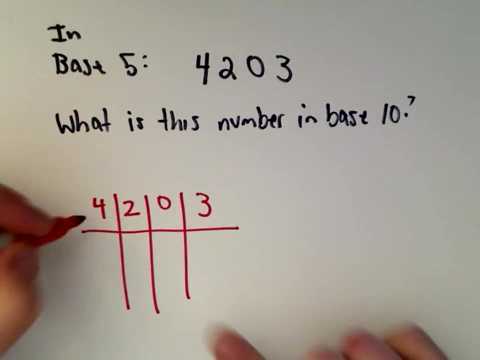 I'm just going to do this little column trick that I did, So we've got 4,, 2,, 0, and 3.. Let's see, So I think I was putting my bases above the numbers, Okay, so here it is, in base 5.. 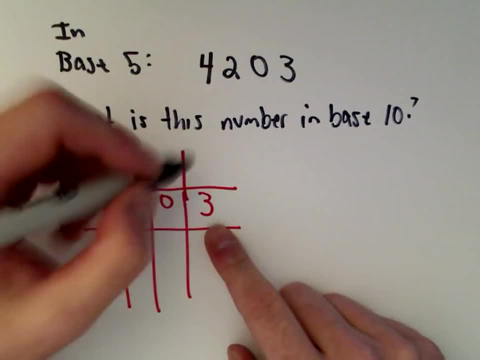 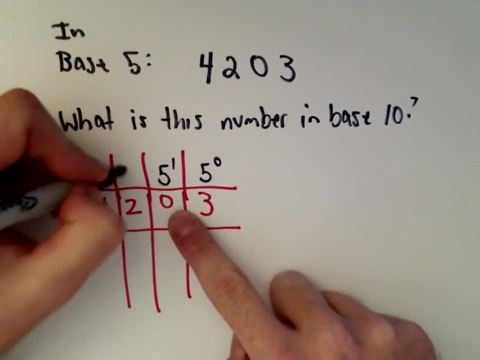 So again, this first digit on the very right that's going to represent our 1's place, the 5 to the 0 power. Then we've got 5 to the first power, 5 to the second power and 5 to the third power. 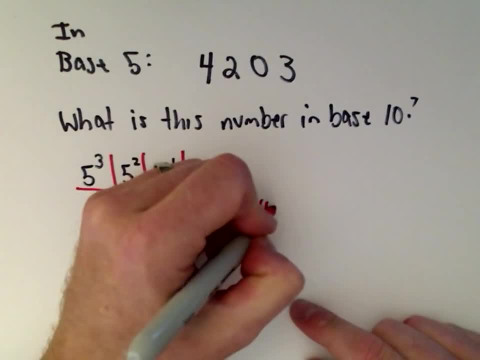 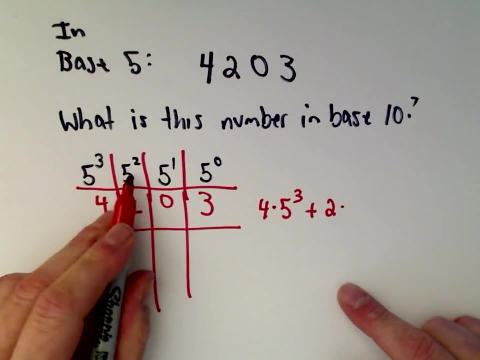 So in base 10, it says we've got 4 of these 5 to the third powers. plus, it says we've got 2 of these 5 to the second powers. Well, it says we have 0 of the 5 to the first powers. 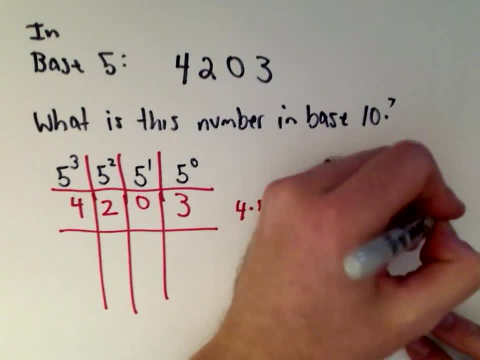 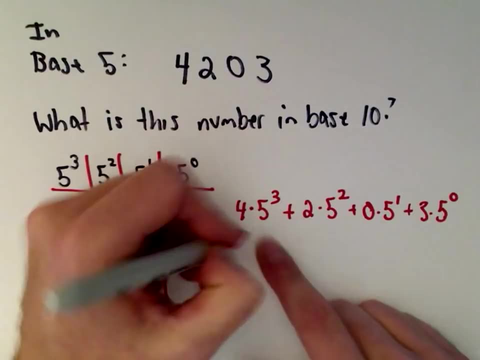 And last but not least, it says we have 3 of the 5 to the 0 powers. Let's see. So: 5 to the third power, recall that that's 125.. So this is 4 times 125. 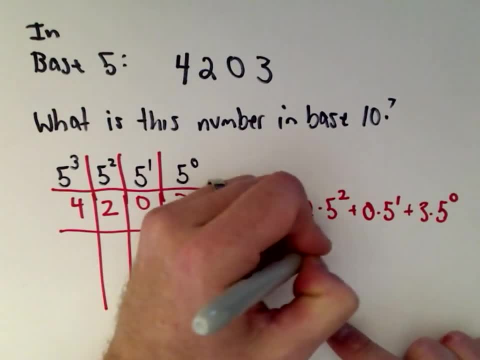 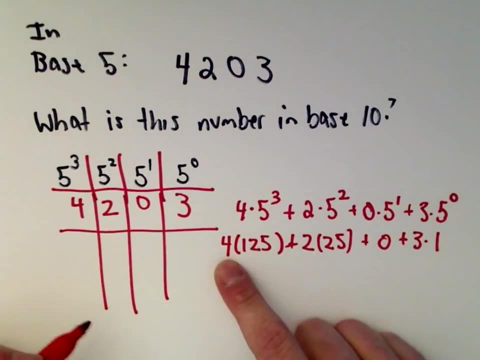 Plus 2 times Well, 5 squared is 25.. Plus 0.. Plus 3 times 5 to the 0 power, which is 1.. So let's see 4 times 125.. I guess that's going to be what 500.. 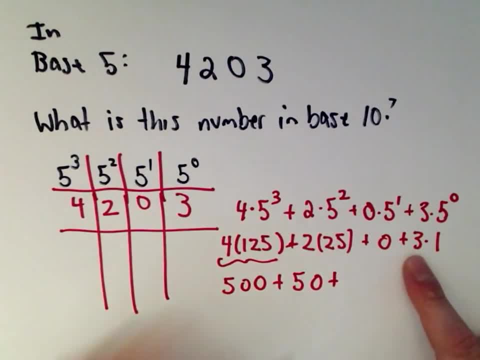 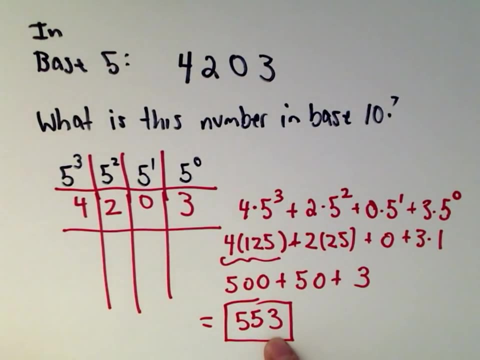 Plus 2 times 25 will be 50.. Plus 0, plus 3.. This would be the number 553 in base 10.. So the number 4,, 2,, 0,, 3. And base 5 would be equivalent to the number 553 in base 10.. 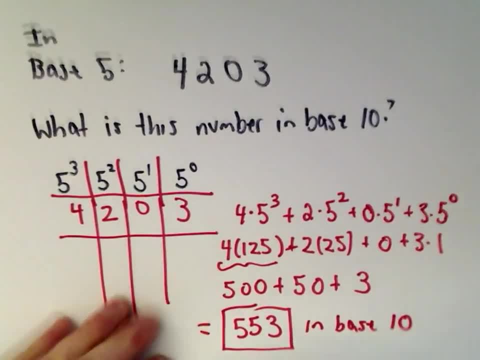 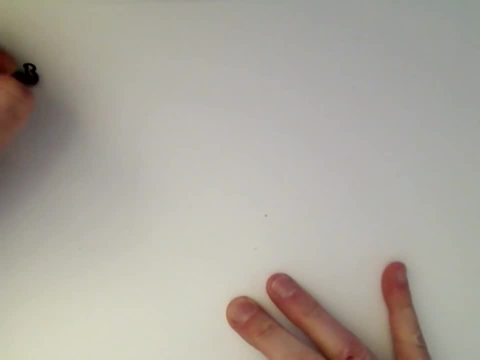 Okay. So let's jump now. Let's do one more. Let's look at base 12 now. Maybe we'll just do one more example of this. So base 12.. And base 12 actually has some interesting uses. 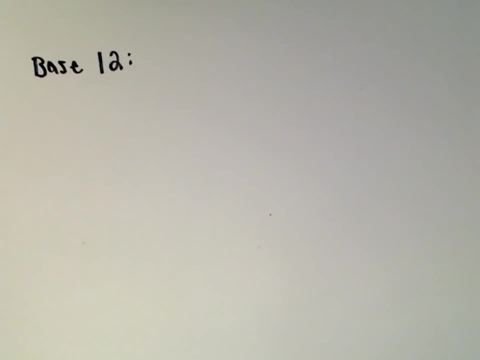 There's some pretty fairy arithmetic that's related to all this stuff, Which, again, I don't know that many people probably need this in their real life, But if anyone's interested in seeing more, I would love to try to understand it a bit better myself. 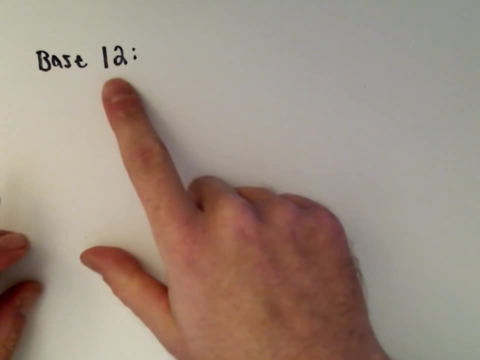 So okay, Base 12.. So okay, We said, whatever base you're using, you have to use digits that are smaller than that. That was kind of what I was trying to allude to at the beginning. So for base 12, we're going to use the digits 0,, 1,, 2.. 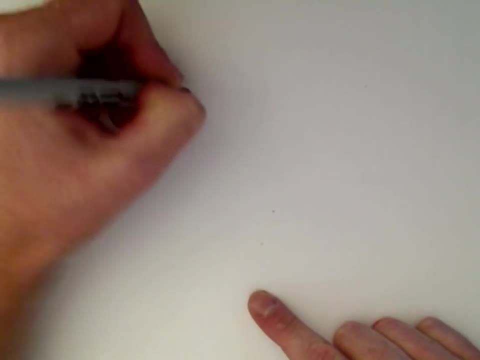 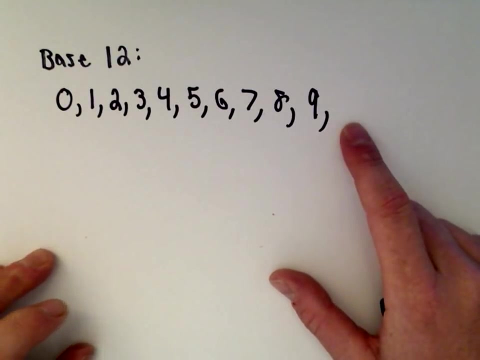 3,, 4,, 5,, 6,, 7,, 8,, 9.. Now I can't write 10, because 10 only makes sense with our base 10.. We need a new symbol to represent the number 10.. 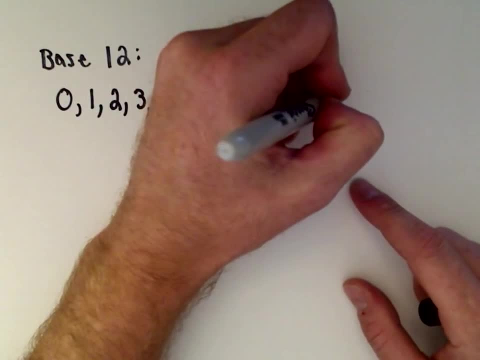 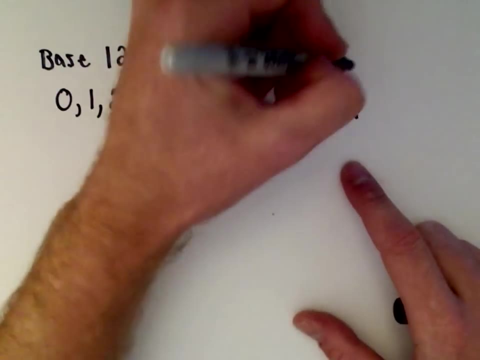 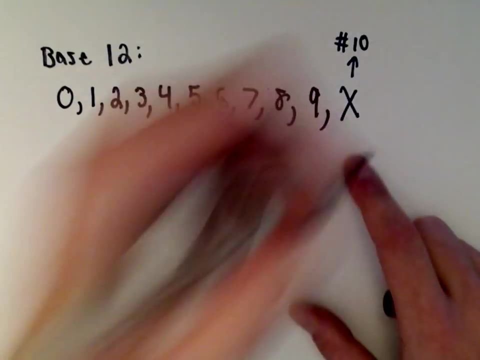 And there's actually some different symbols that people use. One of the symbols they use is like an X, Which you know, if you remember, from Roman numerals. the X represents the number 10.. This represents the number 10.. This is going to be our familiar equivalent, number 10.. 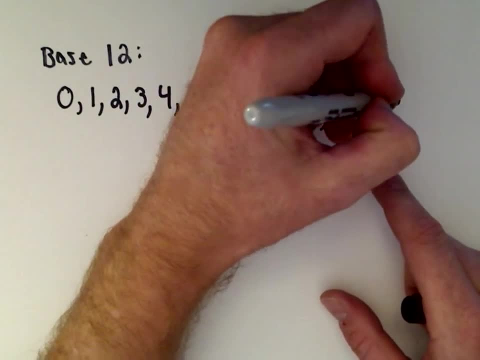 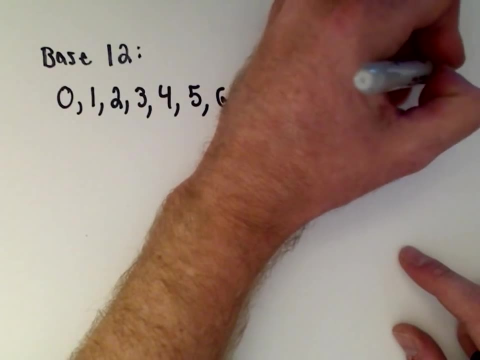 To get the number 11, again, there's some different ways they write it. I think the way let's see the way that I saw them using it it was an upside down. Let's see Which one was it. 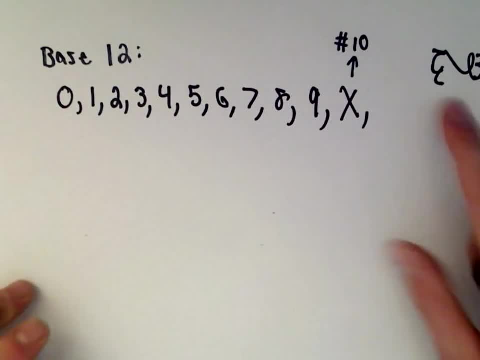 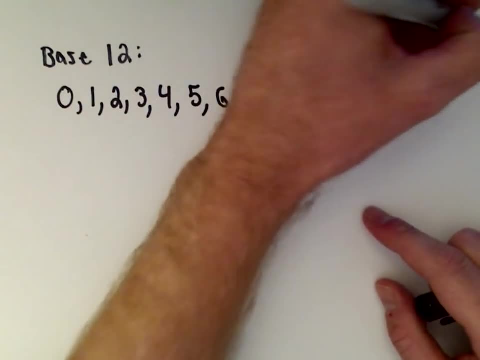 Oh no, I've forgotten now. Oh no, I forget what they used. I should have wrote this down somewhere. They either used an upside down 2 or they were using an upside down or a twisted 3.. I think it was the upside down 2.. 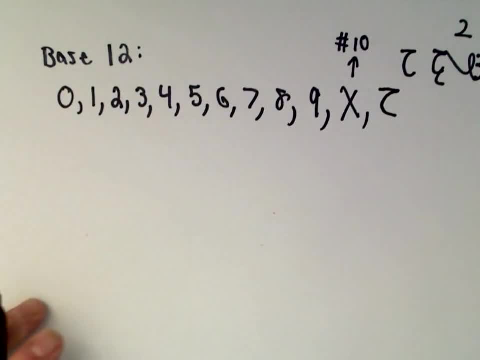 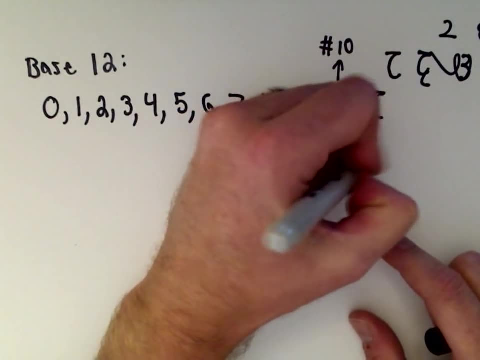 So that's what I'm going to use here, Just and hopefully I'm going to. this is correct. So again, there's some debate on this. Certainly go check this out. I think this is what they use. 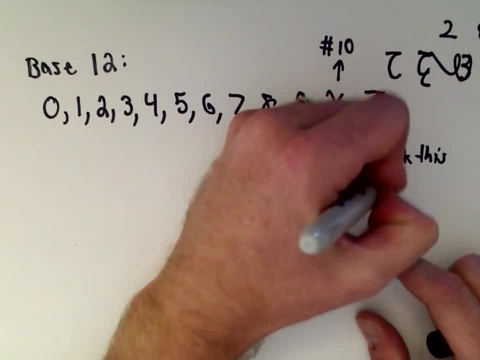 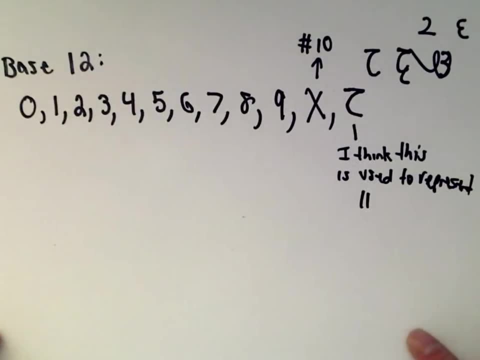 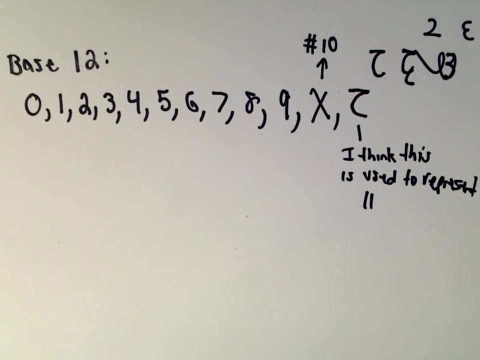 I think this is used to represent 10, or, excuse me, 11.. I had it and then I forgot it. I was looking at this yesterday. So you can double check this. It doesn't matter. I mean, it doesn't matter if you're really interested, but that'll be kind of a minor detail. 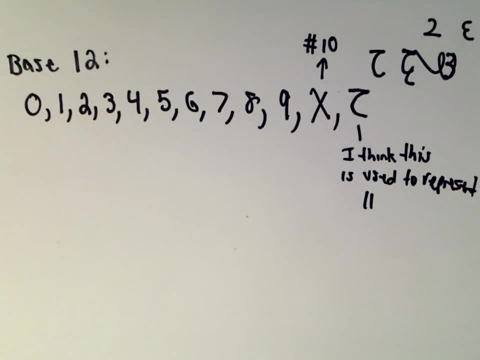 So let's look at maybe one more example. Let's convert. Let's do one last example. Let's convert. So suppose we have the number. So the following number is in base 12. And we want to know what number this is when we convert it to back to our familiar base 10.. 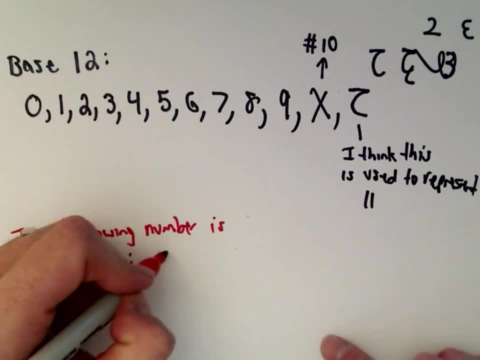 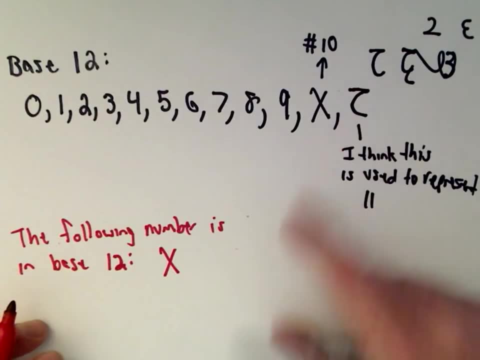 So let's just pick out some numbers at random. So let's use the new symbols, right, because those are kind of exciting. So there's the X, And again, I forgot even what the names of these symbols are. 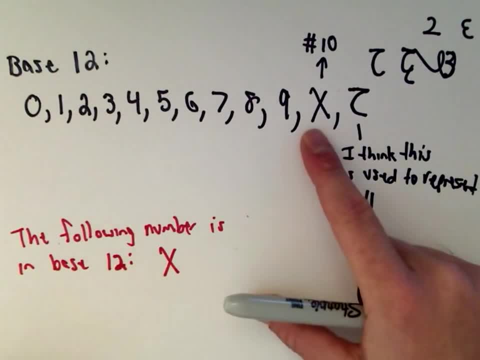 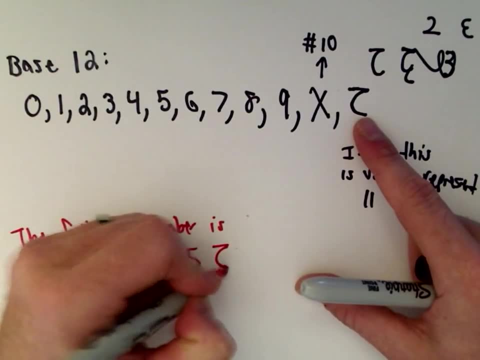 So I'm just going to call it X and upside down 2.. So let's throw an X in there. Let's suppose we've got a 5, our familiar 5.. Let's throw an upside down 2 in there. 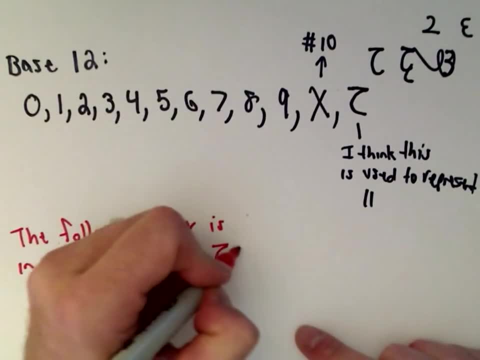 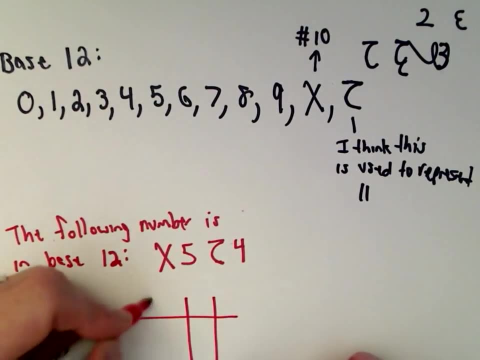 And let's throw one more digit in there. How about? I don't know how about 4?? Okay, So same trick. I'm just going to write down the powers of 12.. And there's definitely proponents for using base 12.. 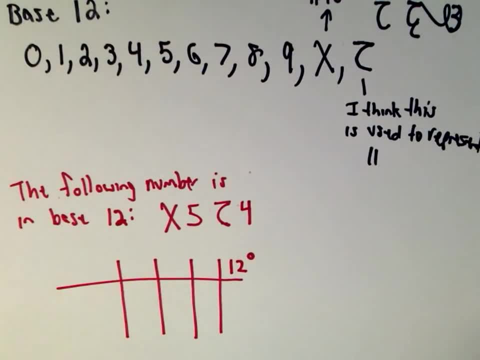 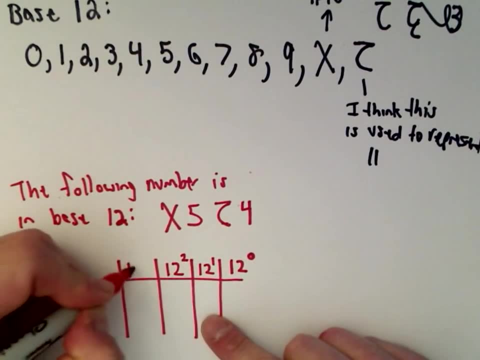 There's actually a whole society. there's a whole group dedicated to using base 12 in the United States and elsewhere around the world. I didn't know that. So there are some big advocates for base 12.. Okay, So we've got our columns. 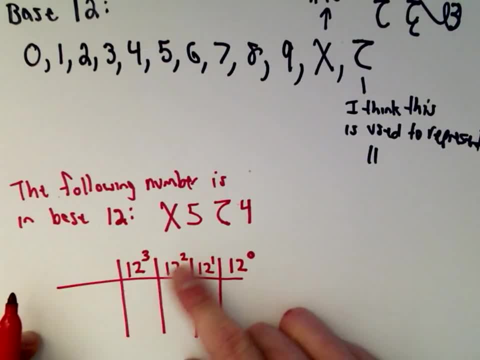 We've got our numbers. We've got 12 to the 0 power, 12 to the 1st power, 12 to the 2nd power, 12 to the 3rd power. So there's our X, our 5,, there's our upside down 2, and there's our 4.. 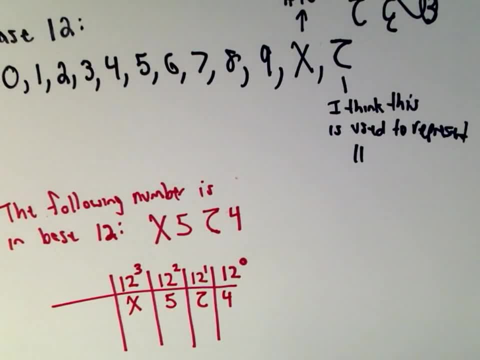 So let me put this off to the side. Let's see What is 12 to the 3rd? I don't even remember that number. I've got my calculator off to the side here. So let's see, Maybe I should know that. 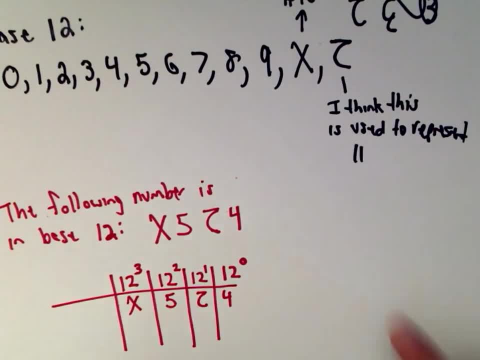 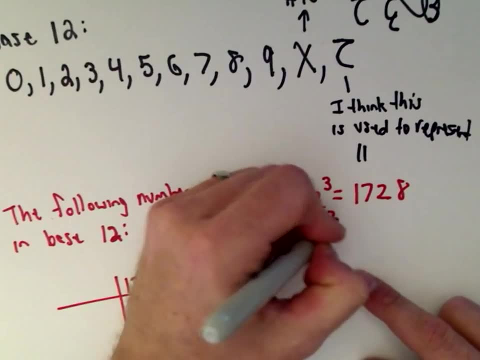 So 12 squared, I know that. one, That's 144 times 12.. Let's see: 12 to the 3rd power, that's going to be 1728.. 12 squared, that's 144.. Well, 12 to the 1st, that's just 12.. 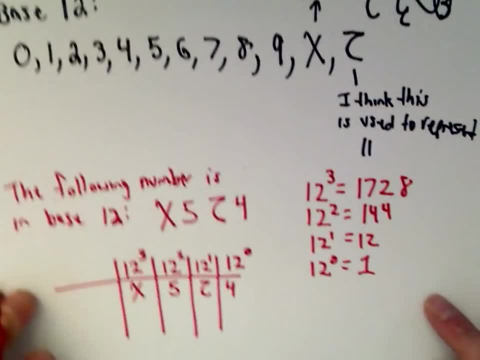 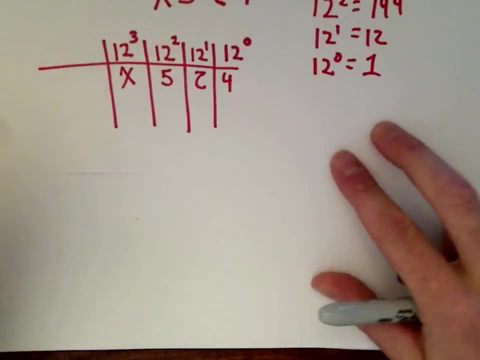 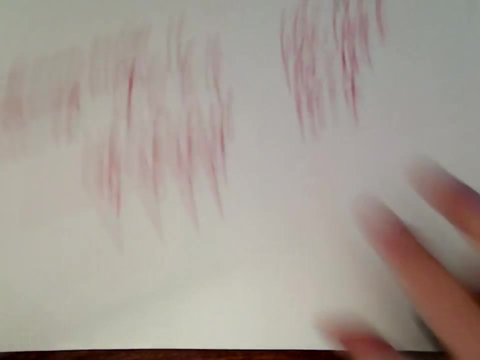 And 12 to the 0 power, that's just going to be 1.. So when we rewrite this number now in base 10, so let me find one more piece of paper- So in base 10.. Okay, So our V here, our X. 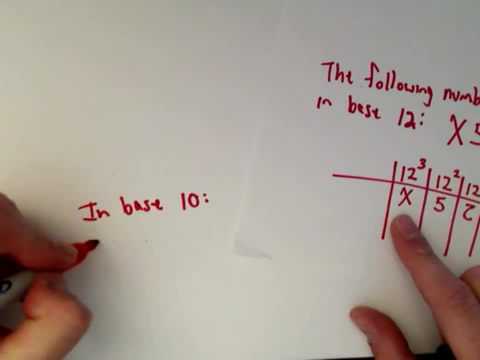 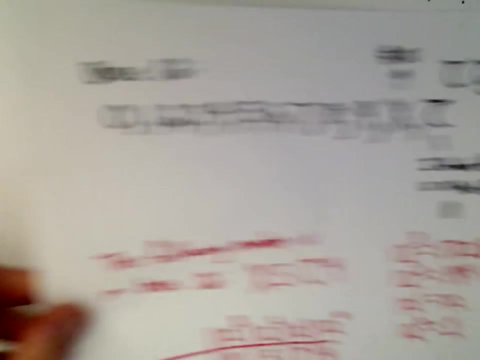 We said that's going to represent our familiar number 11.. So it says we have 11, 12 to the 3rds plus. our next number here was 5.. So then it says we have 5, 12 squareds plus. 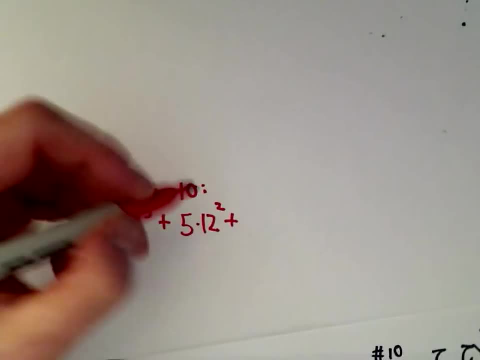 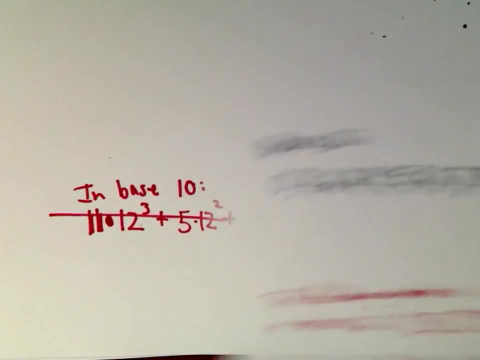 Then it says we've got our upside down 2, which represented the number. Oh shoot, Okay, Sorry, sorry, sorry, I got ahead of myself. Our X represents 10,, not 11.. Excuse me, So let's do this one more time. 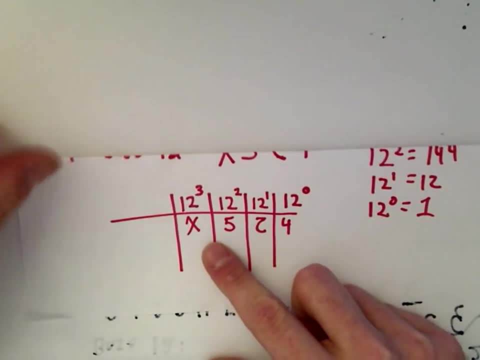 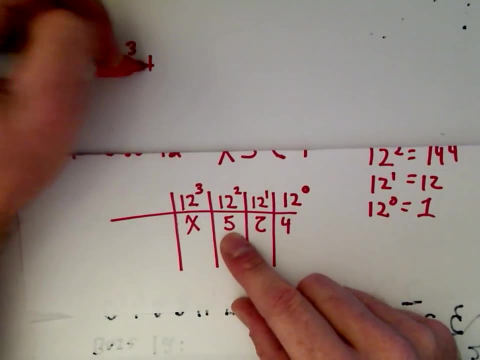 That's why I wrote them out. I'm not familiar with these symbols. I should again remember the X at least. So it says we've got 10 of our 12 to the 3rd powers, plus 5 of our 12 to the 2nd powers, plus. 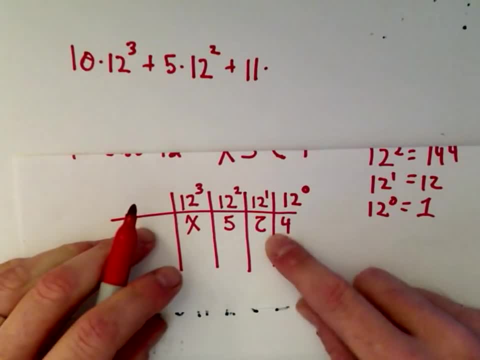 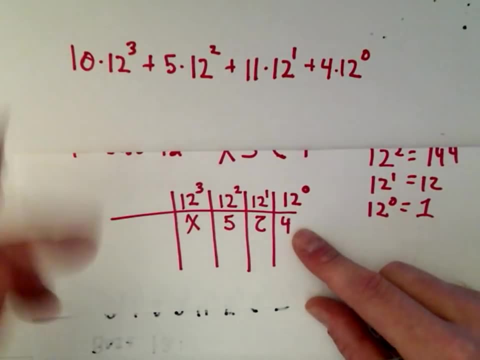 Okay, Our upside down 2, that represents 11.. It says we have 11, 12 to the 1st powers, And then it says we have 4 of our 12 to the 0 powers. So okay. 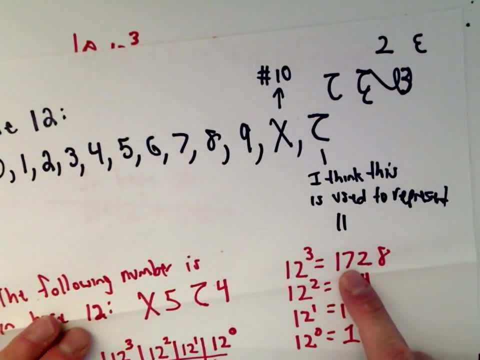 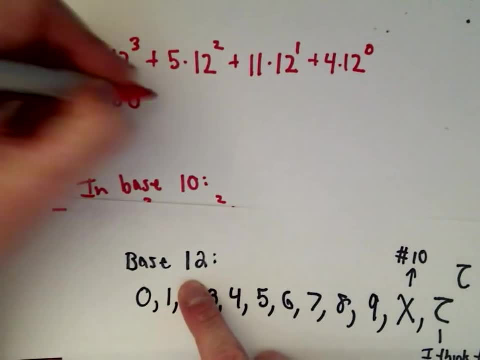 So we said 12 to the 3rd power. That was 1,728.. So if we multiply that by 10, we're going to get 17,280.. Let's see. So we said we've got 5, 12 squareds. 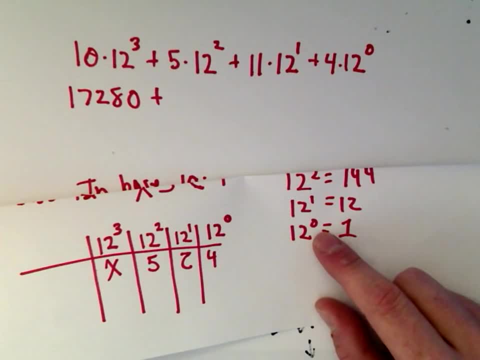 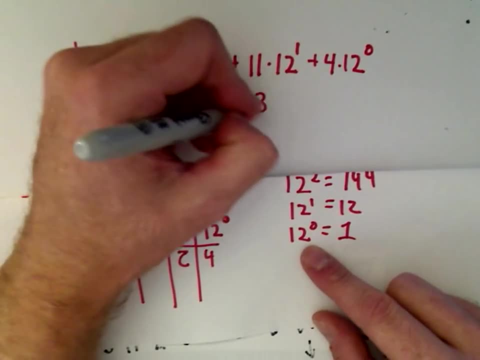 So let's see 5 times 144.. I'm going to again do this off to the side: 5 times 144.. That's going to be 720.. Let's see 11 times 12.. That's 132.. 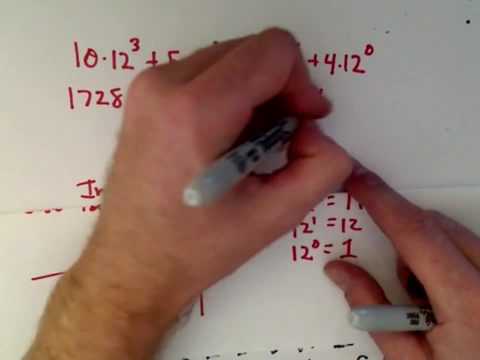 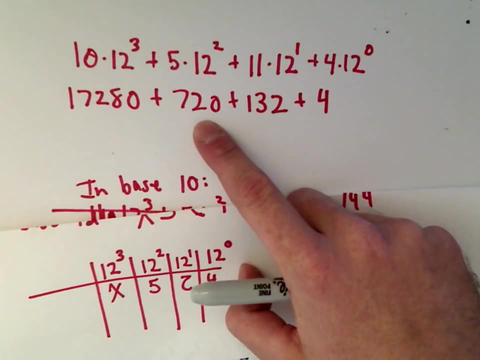 And then we have 44. And then we have 4 times 12 to the 0,, which is just going to be 4.. So again, I'm going to be lazy here- So 720 plus 1,780, plus 132,, of course, plus 4.. 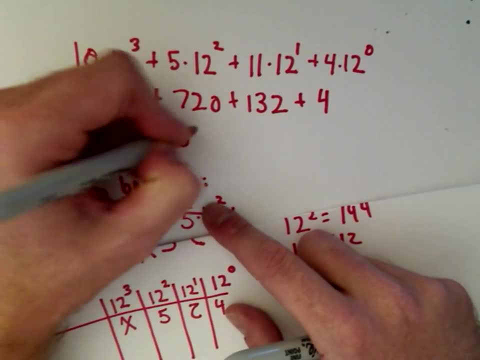 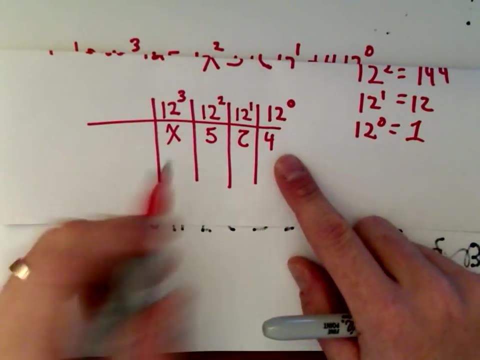 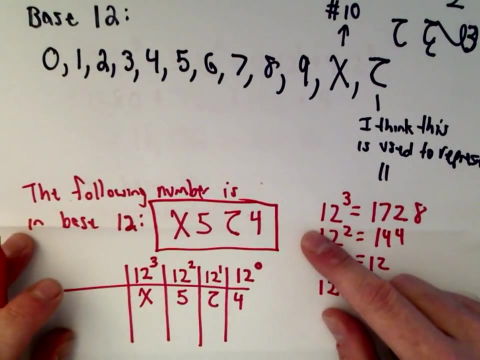 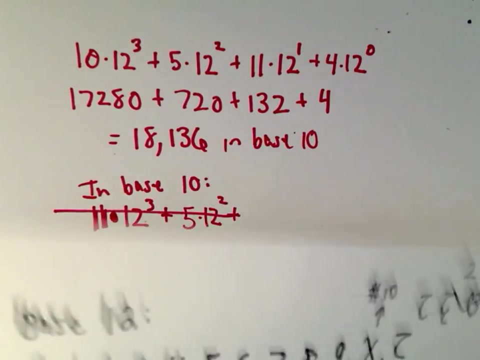 I shouldn't really need a calculator for this- 18,136 in base 10.. So again, this number which was in base 12.. This number which is in base 12, is now going to be equivalent to the number 18,136 in base 10.. 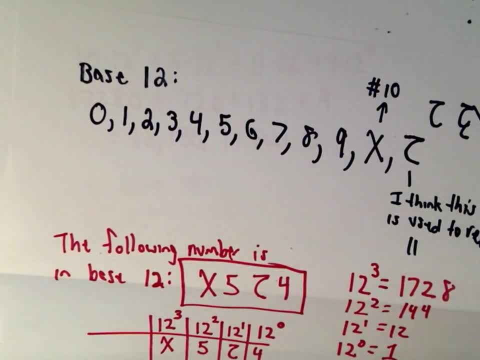 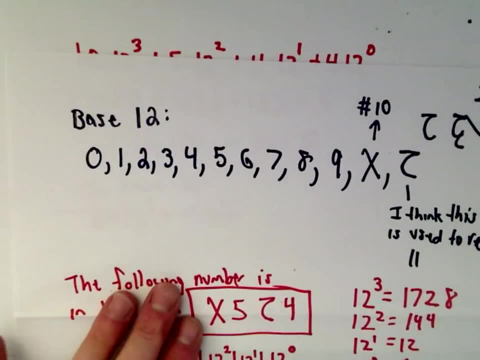 So, okay, I think I'm going to leave it there. Hopefully you see the general idea of how to convert from a number in one base into base 10.. We only did one example where I wrote a number in base 10 into the other base. 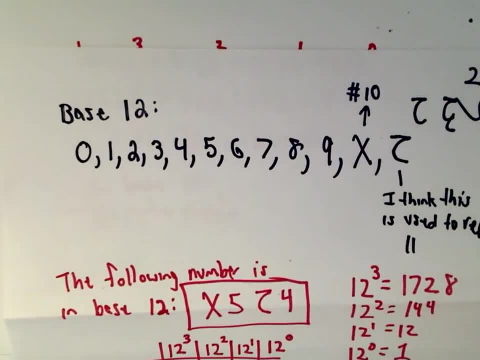 And that was the one using base 2.. But if you need to see any more of those, let me know. I mean we can do some of those pretty quickly. But again, it's basically that idea of you're trying to find the largest power of the base that will go into that number without going over it. 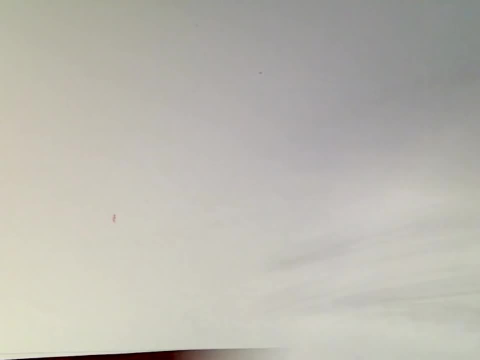 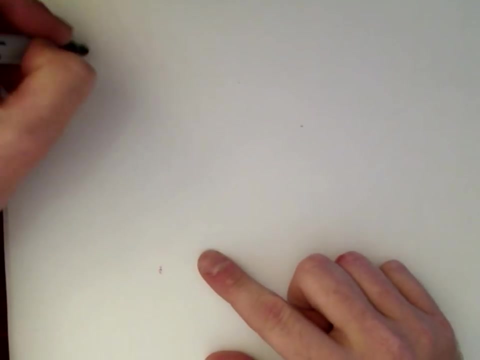 You know what? Let's do one more. Let's do one more because it's fun. So let's write just to be complete here, because otherwise I'll feel like I've left something out. Let's write the number. Suppose we have the number. 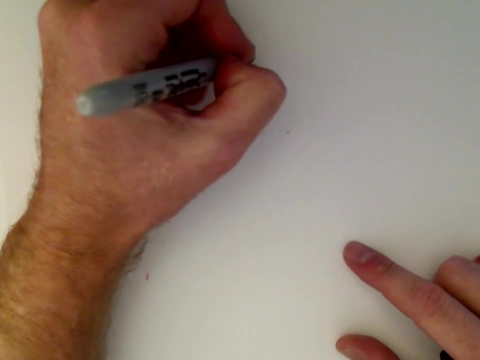 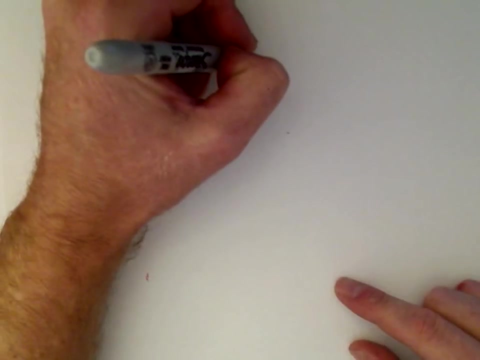 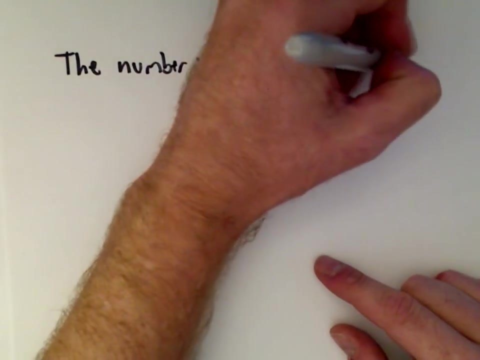 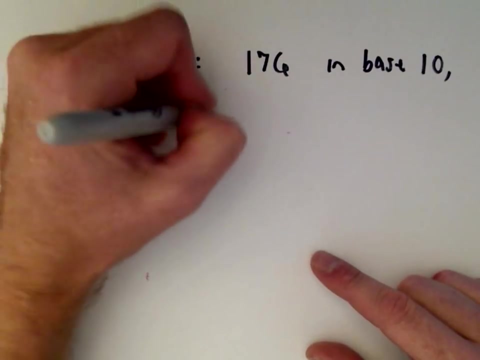 Let's see, Let's use the number. Let's see What's a decent number, I don't know. Let's use 176.. So the number 176, and suppose that's in base 10. And let's write it in base 5.. 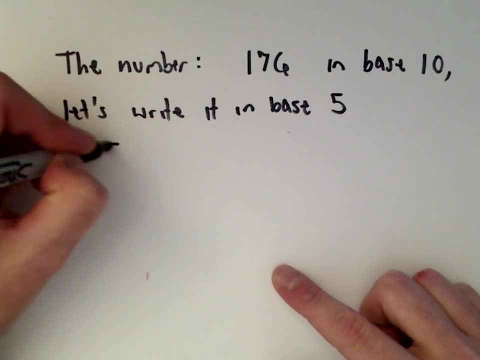 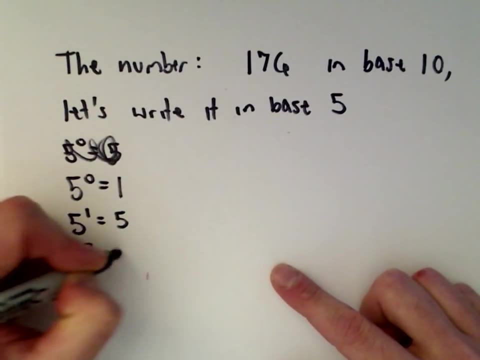 Okay, So again, 5 to the 0.. That's going to be 5 to the 0.. That's going to be 1.. 5 to the first, power is 5.. 5 squared is 25.. 5 to the third is 125.. 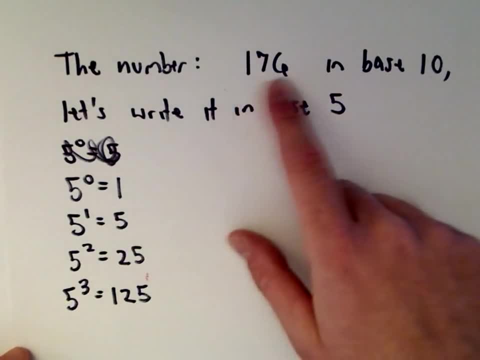 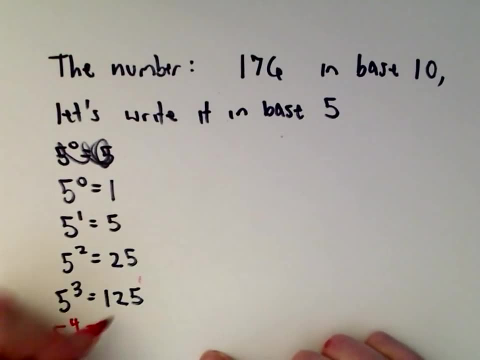 And any power larger than 5 to the third is definitely going to be bigger than 176.. So I'm going to do the same thing. I'm going to think, okay, Right, Because once we get to 5 to the fourth, if we multiply that by 5, what is that? 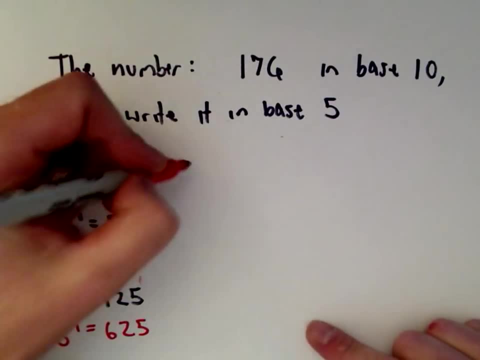 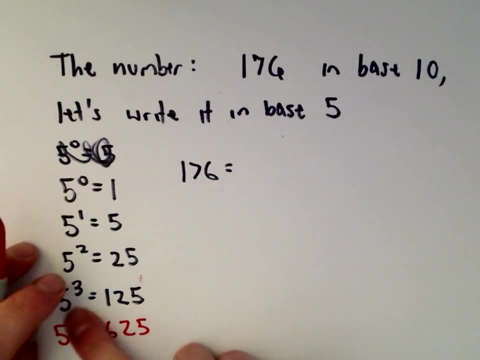 625.. Okay, We're already too big, So 176.. The largest power of 5 that will go into that is 5 to the third. So I would need 5 to the third And I'm going to do the same thing. 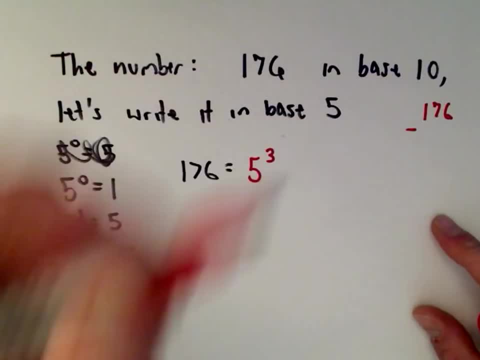 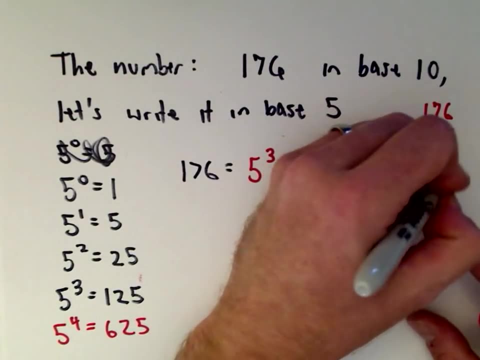 I'm just going to subtract, So 176.. If I subtract away 5 to the third, which we said is 125, that's going to leave us with what? 51.. Okay, So now I do the same thing. 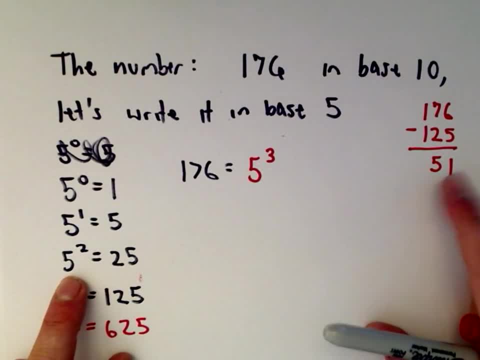 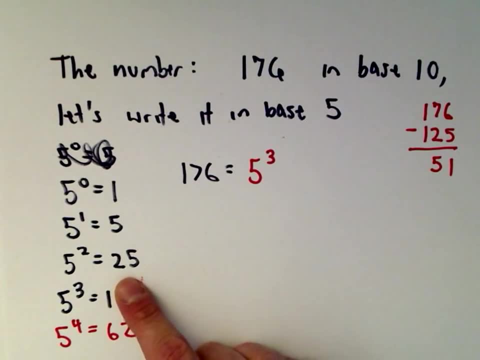 I think what's the largest power of 5 that will go into 125? 176 without going over? Well, it looks like 5 squared is going to be the next one, But notice, we can actually use two multiples of 5 squared. 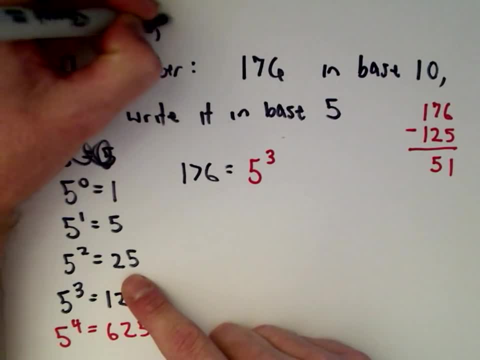 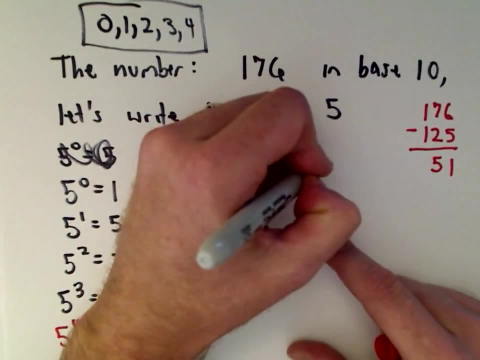 So I can only use the digits 0,, 1,, 2,, 3, and 4 when I write my number using base 5.. But I can actually use two multiples of 5 squared, So two multiples of 5 squared.